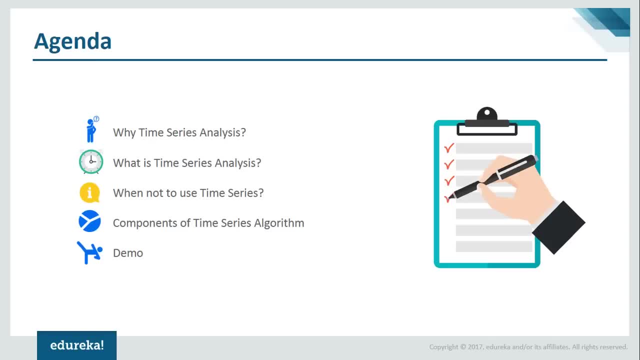 to scare you with scary maths today, But I just want to get an idea at what extent I have to explain the concepts today. So can you please confirm me in the comment box with your reply? So I repeat: are you guys familiar with a few of the concepts of maths, such as what is mean? 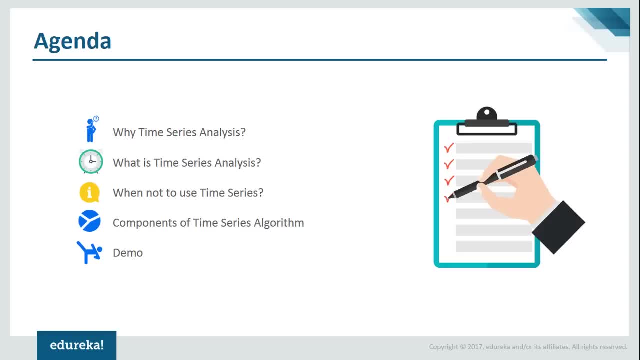 what is variance, What is covariance Right, And how many of you are familiar with the data science background? Alright, so I can see that Avinash is saying he's clear. So is Ajay Manish, Avinash Right. 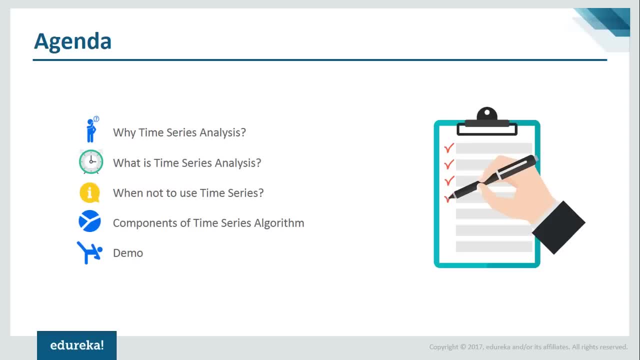 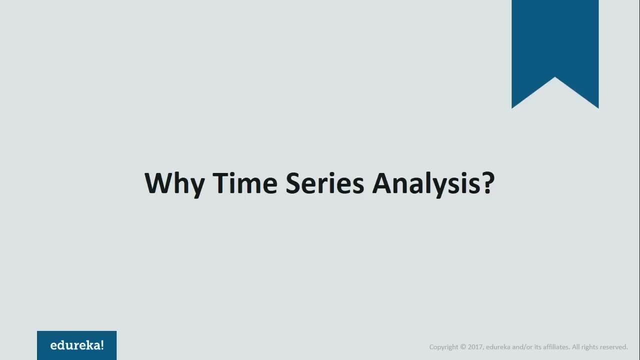 Avinash says: absolutely. I like your confidence, Avinash. Alright, so let's move ahead and start off with our session. The first topic is: why do we need time series analysis? So, for those of you who are not Acquainted with data science, There are quite a few algorithms in data science which can predict values right. 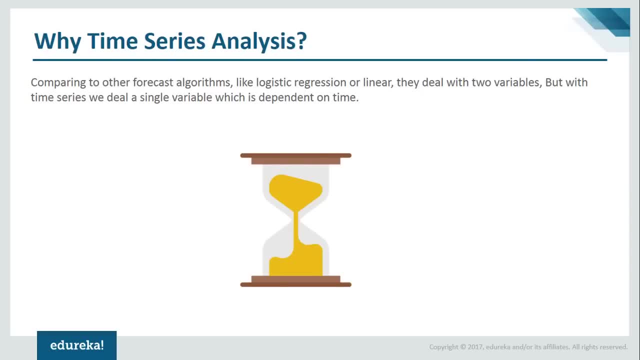 But why do we need one more algorithm called the time series algorithm to predict value? So let's see with that. So, if you would have noticed, in other algorithms, such as the linear regression or logistic regression, There were two variables right, One was a dependent variable and one was the independent variable. 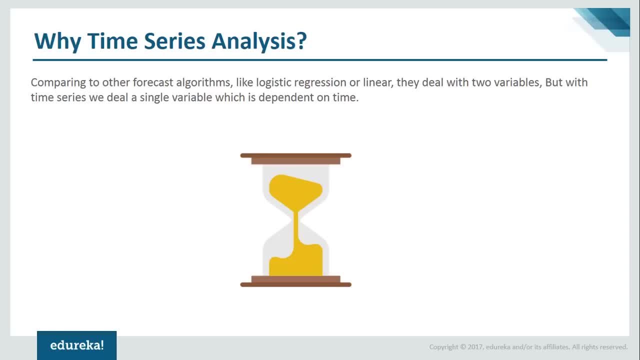 So you used to predict the dependent variable based on the values of the independent variable, for example, a particular value of X. You used to give a particular value of X and you used to see what will be the value of Y. but in time series analysis, the scene is that you will be. 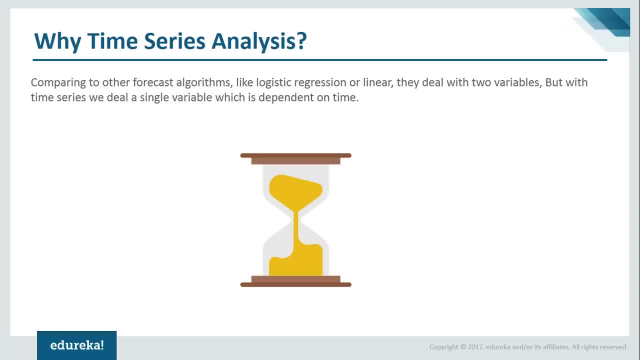 Given only one variable and you have to predict that we in one variable. now Imagine if you just have one variable. how will you predict it? and the only thing which will be given in the data set is In accordance with the time. that is there, right? For example, if I own a company, I own a car company- 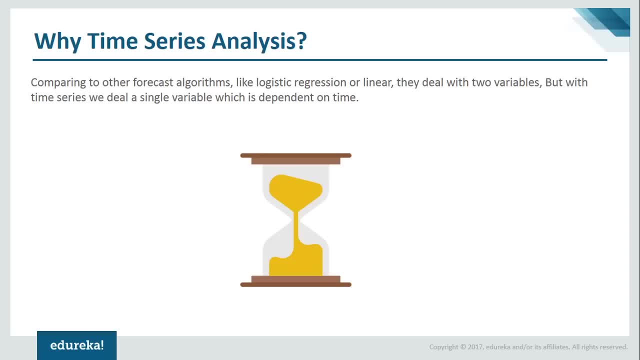 I own a car company and I say that last month I sold around 23 cars. this month I sold 24 cars. What is the sales that I'll achieve in the next month, Right? So in these cases, you would have noticed that the only variable that I have is the sales part, right? 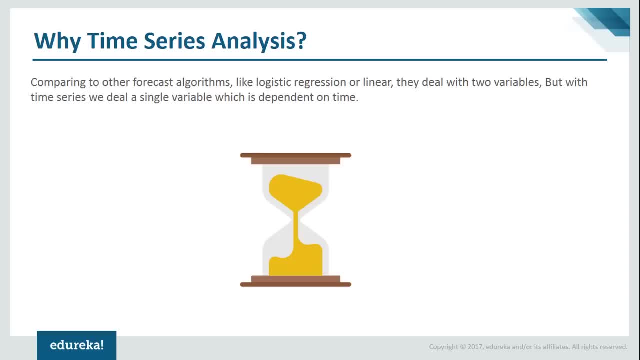 I don't know What is the, So I don't know What is the other variable that I have to depend on. the only thing that is there is time, right, So I have to predict for the next month. So same as the scene here. you use time series analysis when you have only one variable and you have the time. 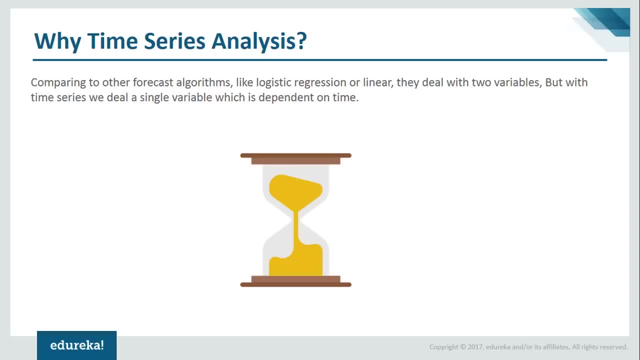 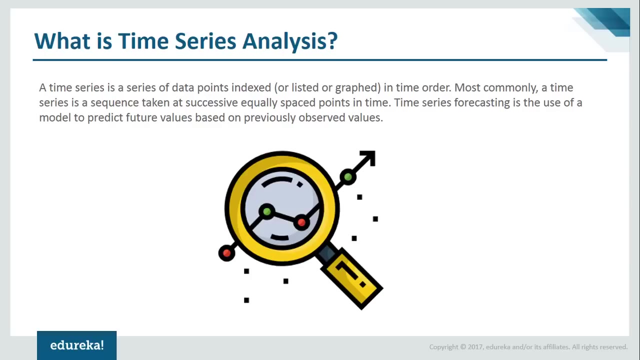 as a second Variable that you will be predicting the value from. Alright, Now, this is why you use time series analysis. Let's now understand what is time series analysis exactly? Alright, so time series is a series of data points Indexed in a time order. Alright, so it's a series in which you have indexed the points according to a time order. 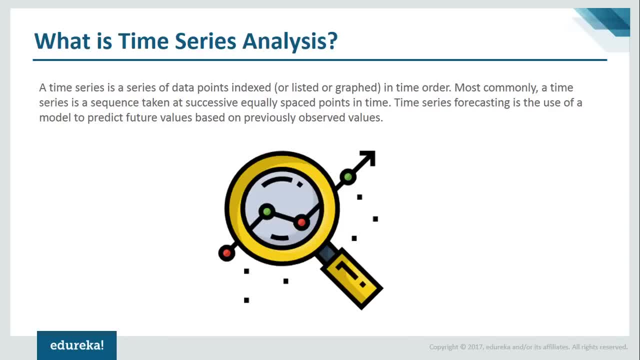 Now you use a time series algorithm to create a model, right, And once you have created that model, you use that model to predict values, Right you? you predict the future values. whatever future values you, you have right, Whatever depends on your use case. So this is what 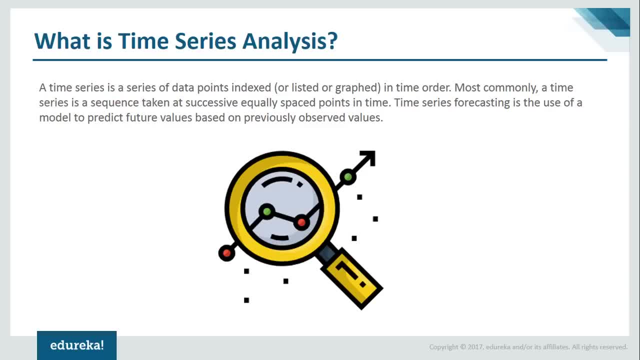 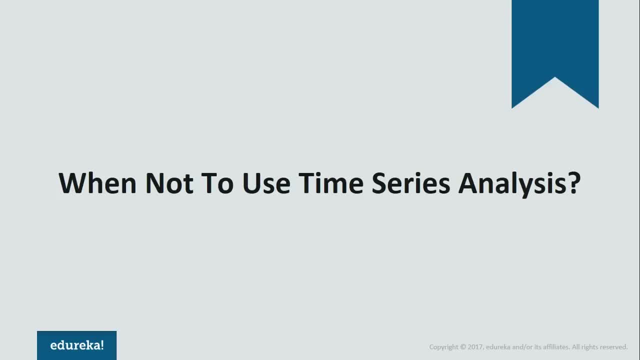 Time series analysis is all about. you create a model, you give it the inputs of the past and you predict the future values. All right, Moving ahead, guys. Now this is where you use time series analysis. So I told you, whenever there is a time component, you use the time series analysis. 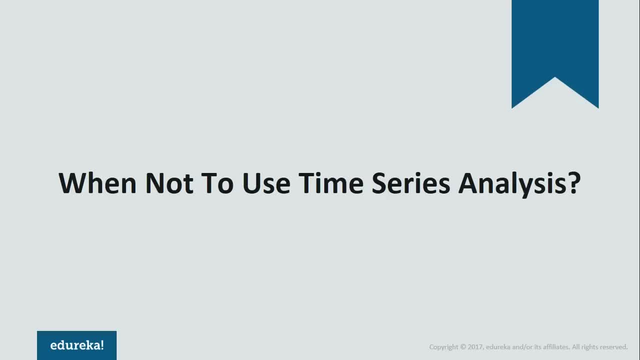 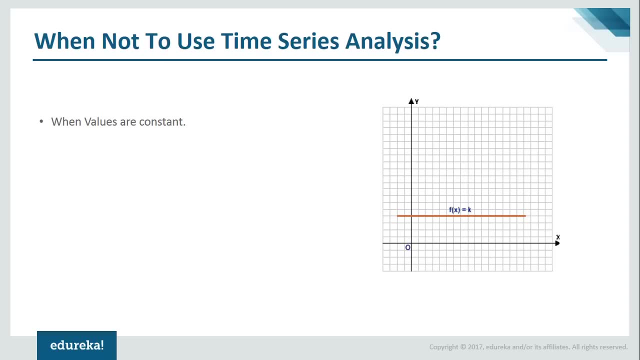 Then where, but when? do we not use time series analysis? So we don't use time series analysis whenever the values are constant, Alright. so, for example, I say that my company sold 23 cars in the past month, 23 cars in this month. Tell me what is going to be, what is the sales that is going to be in the next month? 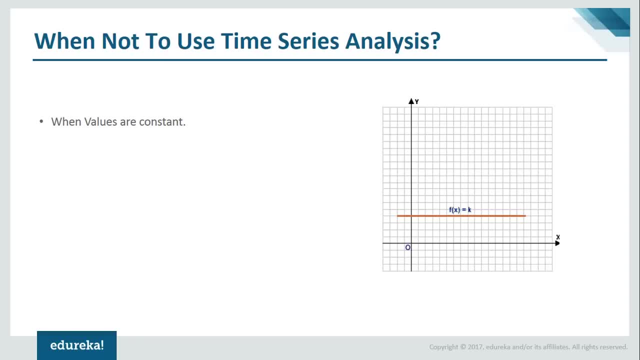 So right. so in this case my number of cars is same for the previous month and this month as well, right? so there is no need of any analysis kind, or there is No point of putting an analysis over there because it's kind of obvious. and if, even if it is not obvious, maybe 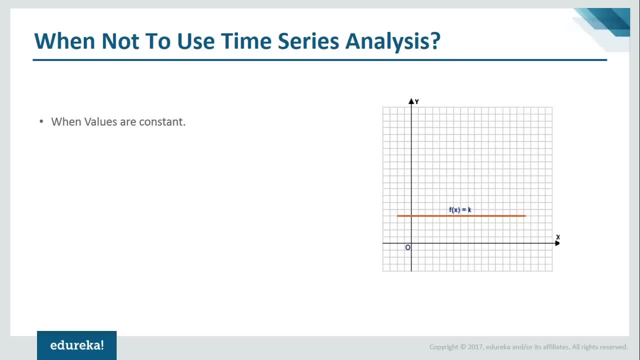 There is something that is Going to be there next month, Maybe there's going to be a discount next month or something like that. But all of those parameters if you cannot include in your analysis, there's no point in putting that analysis right. and Specifically time series analysis, because it was all dependent on time. 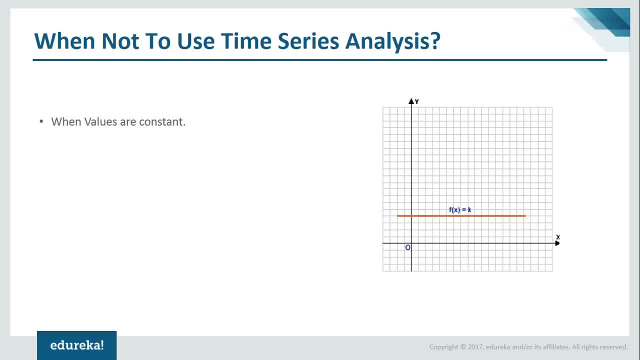 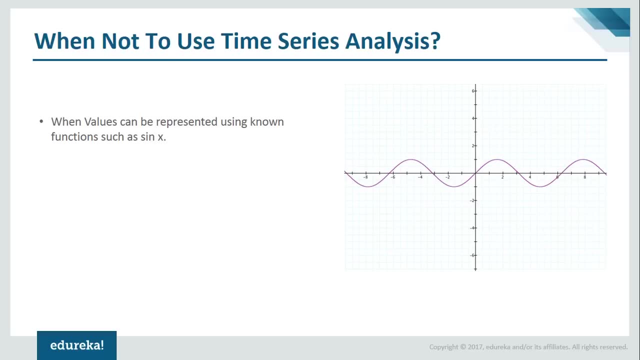 Having said that. so, like I said, if values are constant, you cannot use time series analysis. similarly, you cannot use time series analysis if you have, If your value is represent, can be represented using a function, for example The sine X function, right, So if you have the X value, you can get that value using by putting it in the function. now, 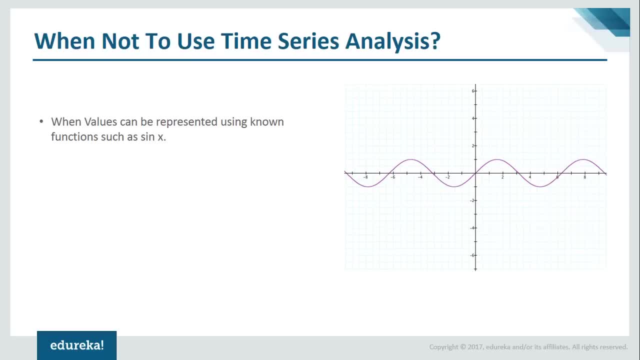 You can apply time series analysis on this as well, But there is no point because you can. you could have got that value by putting it in the function itself, Right, just like the sine X value or the cos X value, or any other formula for that matter, right? 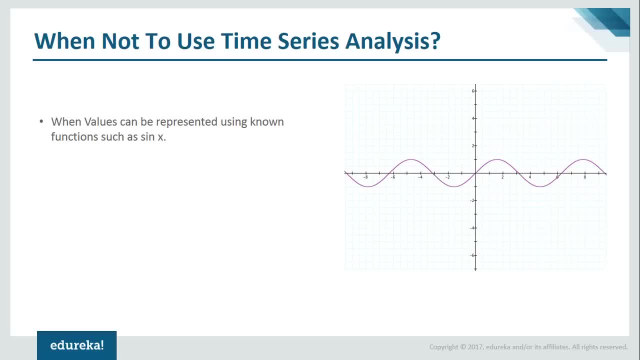 So there is no point in doing time series analysis if you have a formula before that, Okay. Now this is the scene when you should not use time series and all analysis. but what are the cases in which you cannot use time series analysis, in the sense you cannot do time series analysis if 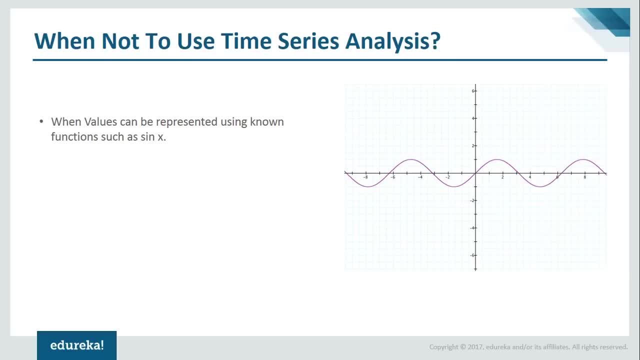 this Data is like that. So there's a concept called stationary. So if your data is not stationary or your data series is not stationary, you cannot apply time series analysis on that. Alright, so what is stationary? So, if so, being for for the series to be stationary. 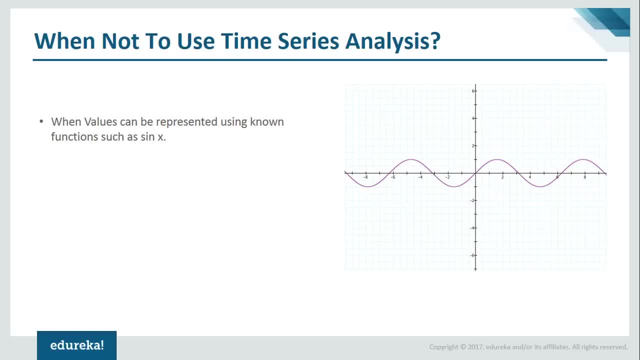 There are three conditions. So the mean should be constant according to the time, Alright, The variance should be equal at different time intervals from the mean. So what now? for those of you so mean is basically the average, right? For those of you who don't know what variance 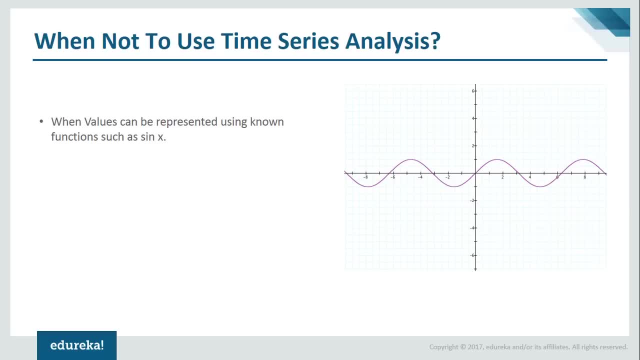 is? it is basically the distance from the mean. So each point distance from the mean should be equal at equal intervals of time, and that is what variance is all about. That is, how far each number is from the mean. Alright, So this is what variance is all about, Then. 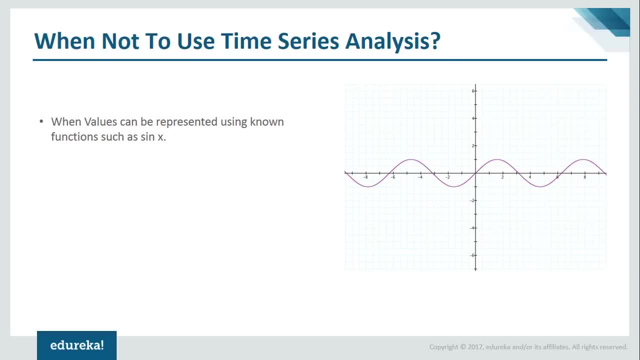 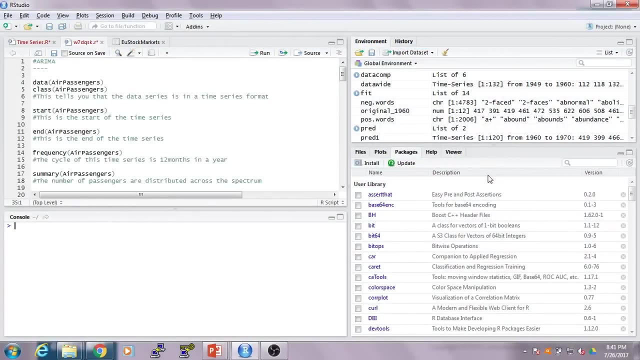 we have the covariance, so that should be also equal. So if these three conditions are met, then only we can say that my series is stationary, and then I can apply the time series analysis. Alright, So let me give you an example. So, guys, this is. 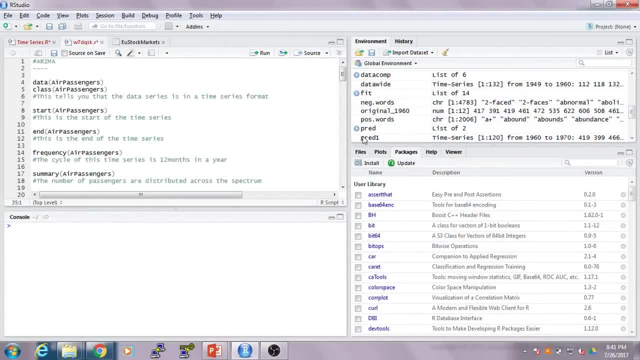 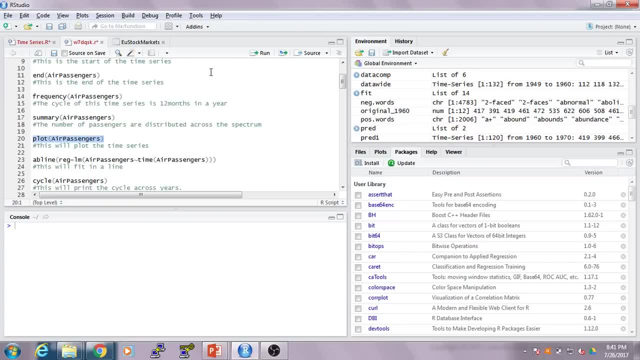 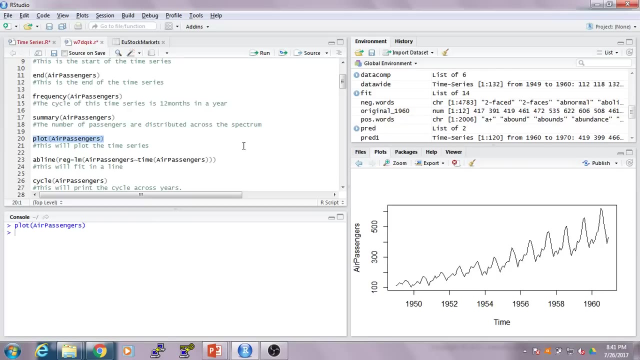 my R console Right Now if I want to find the mean. So let me first show you the data that I have, Right? So this is the graph that my data is representing. So, basically, I'll be doing my time series analysis on air passengers today, Alright, So this is the graph that. 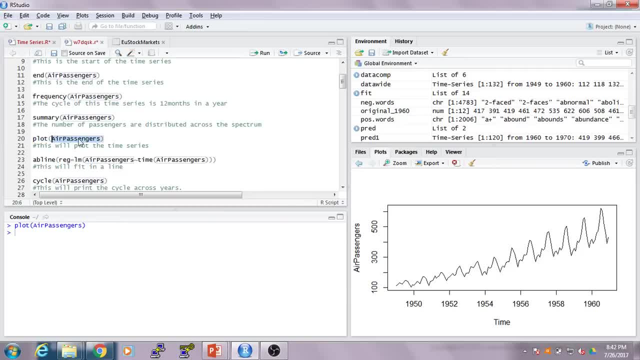 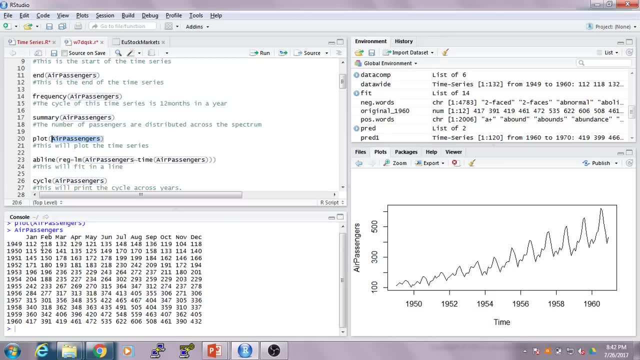 air passengers data has right now and if you want to see the data set, this is how the data looks Right. So we have data from 1949 to 1960 for each and every month and we have to predict for the next 10 years what will be the sales of the tickets. We will do that. 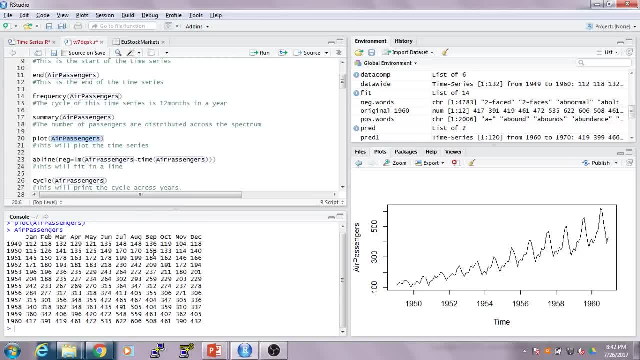 today. Okay, So for now we are concerned with the mean. what is mean? So mean is basically the average of the points. you'll be calculating the average of these two points and you'll be pointing- I'll put a dot here. Similarly, you would put a dot here and you'll pass a. 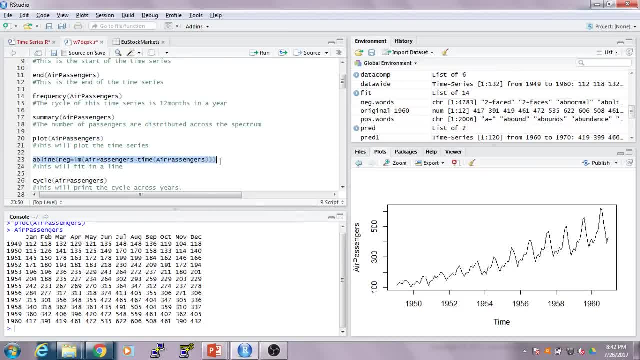 line through. So this is the mean, Similarly, the average of these two points, and you will miscalculate and you put a dot here. Similarly, you put a dot here and you through it. so let me show you how that line will actually look like. now. this is: 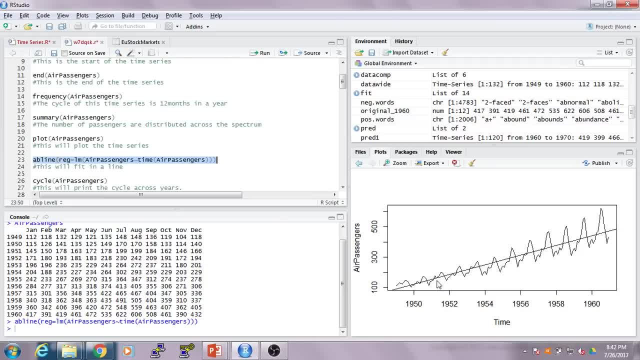 the mean, guys, this is the mean that I've plotted. so, as you can see, the mean is changing according to the time frame. so if I talk about the ears, my mean is changing. right, it is not constant. for example, in 1950 the mean is increasing. 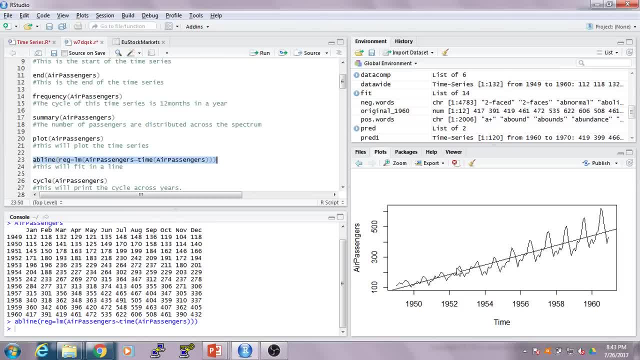 from 1950 to 1952, my means value has increased it right. so this means value should not be increasing. it should, but should be constant. so this we have to look at, and then we let's talk about variance. so variance is, like I said, the 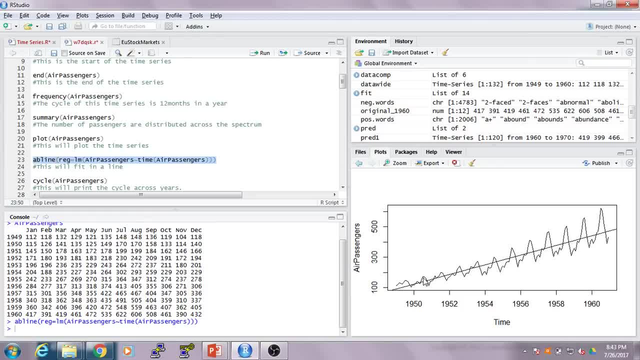 distance of each point should be same from the means. for example, this particular point over here, or let me get a bigger wave. so this particular point and this mean, if this is a distance, distance, then this particular point and this mean should also be the same. but that is not. 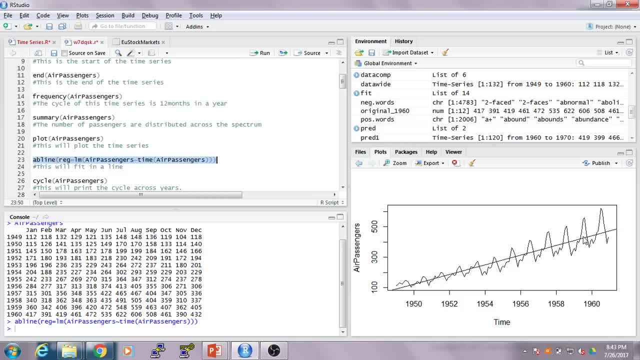 the case right now. so we have to transform a data so that our variance becomes equal. all right, so that is what we are going to do right now. so if my variance and my mean and my covariance, they become equal, my data series become stationary and hence I can apply time series analysis on that. all right, so 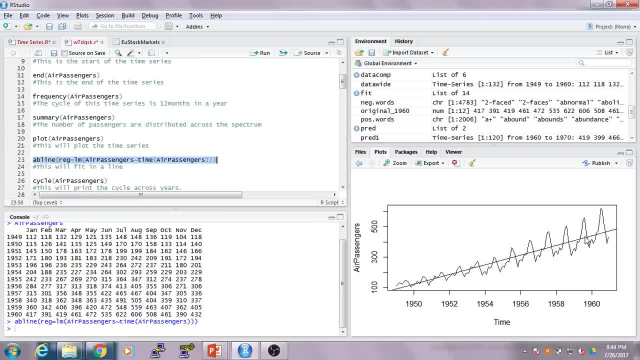 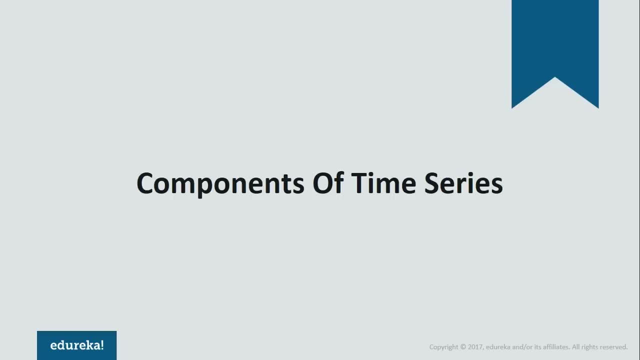 this is the. this is what you should be clear about till now. if you're clear to know the journey head is a cakewalk guys. there's nothing tough to what is going to be there in time series analysis. all right, so let's we've discussed what cases we should not apply time series analysis to. 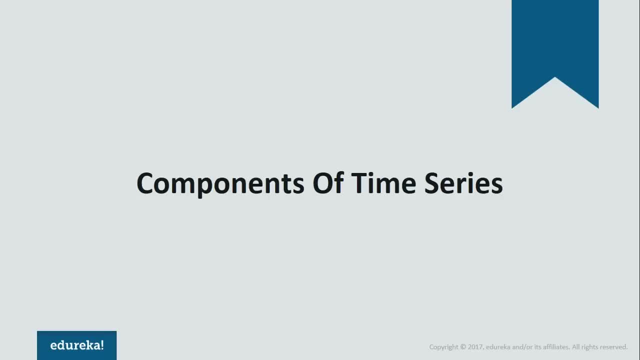 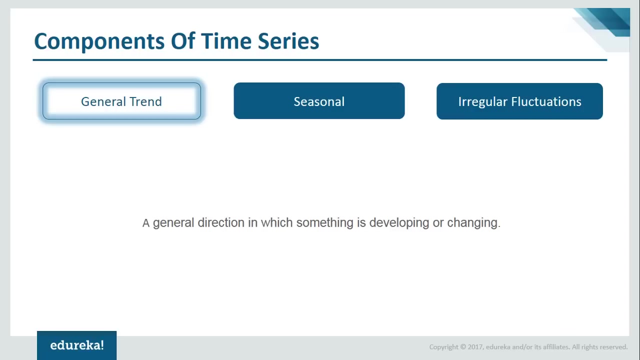 and when. which cases there? there's no point in applying time series analysis. now let's move ahead and understand the components of time series. all right, so when we talk about the components of time series, guys, there are basically three components. you have the general trend, then there is seasonal and there are irregular fluctuations. so let's discuss these. 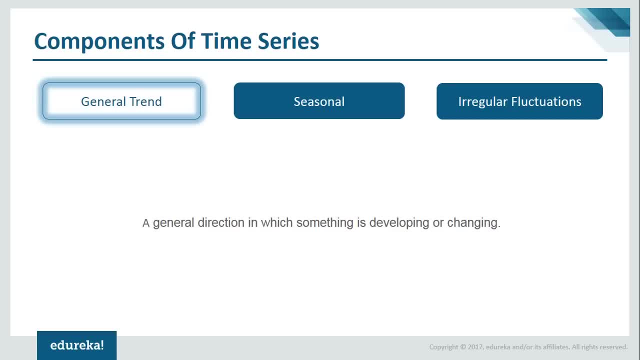 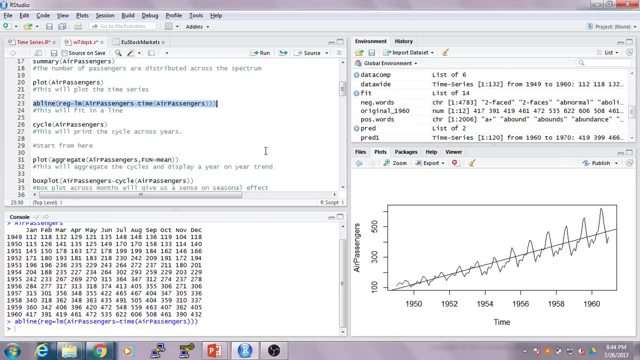 three components in detail. so the first thing is the general trend. so a general trend is basically: how are your values going? are they increasing or are they decreasing? all right, so let me give you an example by showing a graph. so let me go back to my our console and let me give you a trend. 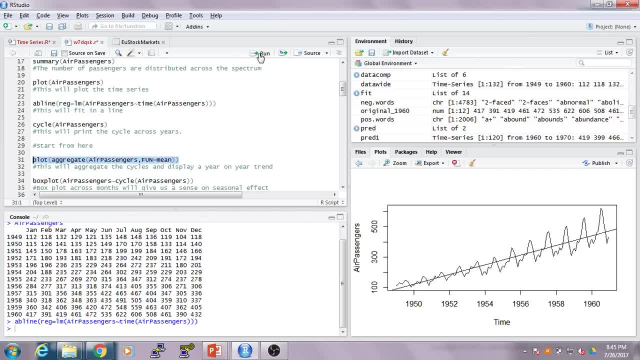 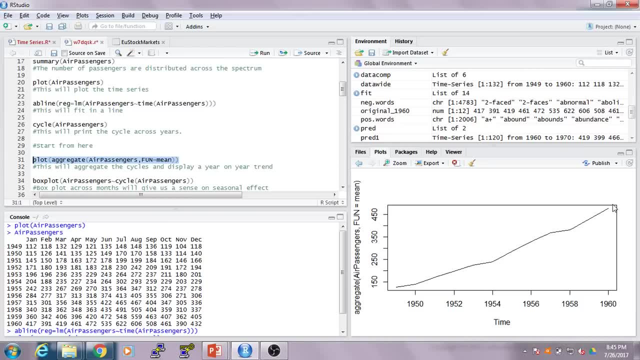 all right. so, guys, this is the trend that my values are going through, that is, my values are increasing every year and that is how the trend is going. now, my trend can be either upwards or it can point downwards- all right, and it's a component of time series. now you can see that. 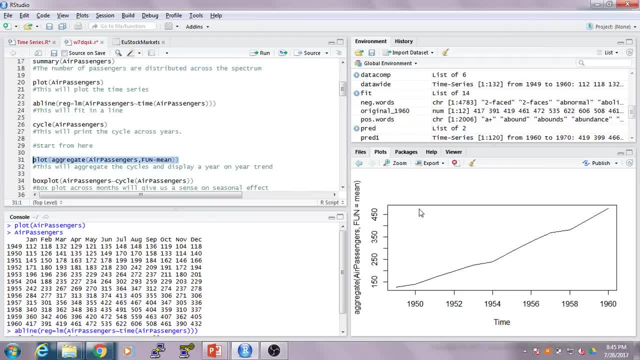 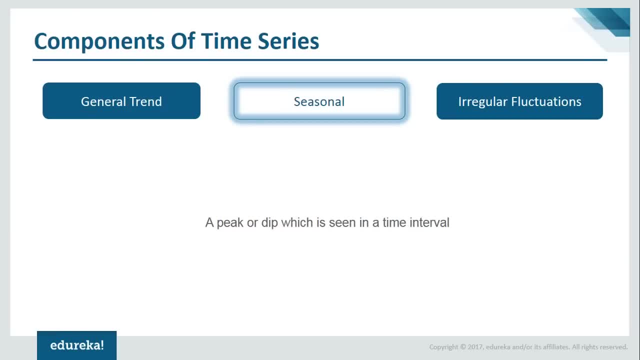 in the data set as well that my values are increasing and hence the trend is going going upward. all right, so pretty simple. this is what general trend is all about. and then we have seasonal. so what is seasonal data, or what is the seasonal component? so a seasonal component can be. 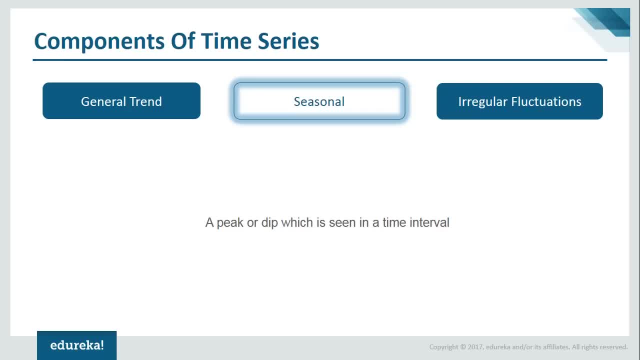 understood something like this: so you have an airline company right now, you would have noticed that at every festival, there is going to be a peak in the number of commuters that are going to take your airline. for example, near christmas, a lot of people will be going home and hence there will be 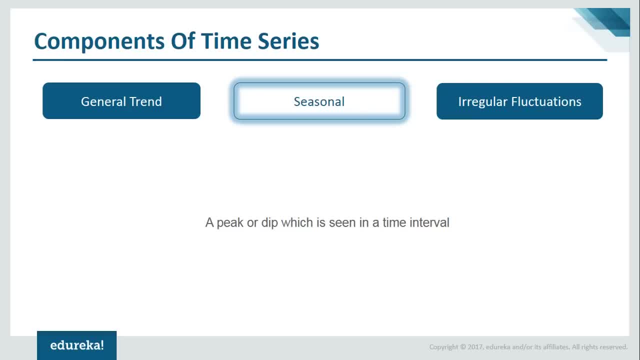 a spike in your uh in in the number of people who will be traveling through your airline and hence you would have also noticed that the number of people who will be traveling through your airline. you would have also noticed that whenever you try to book your tickets in the peak times, that is. 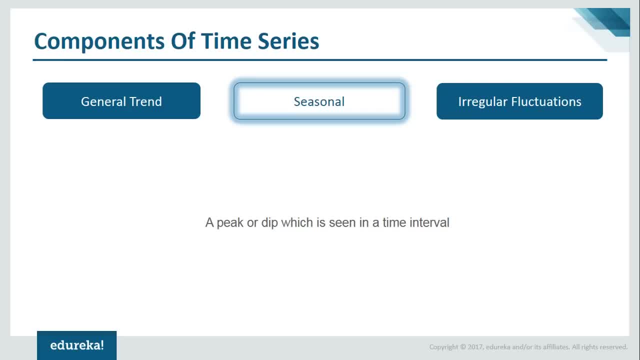 during diwali or during christmas, that the fears are quite high. and they are high because the airlines, they have already speculated that at this particular time, my number of passengers would be more and hence there, and it is imperative for you to go home right, and it doesn't matter how much. 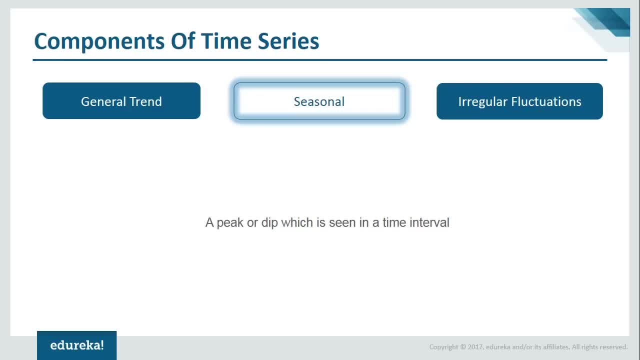 cost they are asking you, and hence, that is the time that the airline makes the maximum profit, right? so this is the trend that i am going to talk about in this particular video, and i am going to talk about the seasonal part of the year, so this is the seasonal part that i am talking about. so, in a 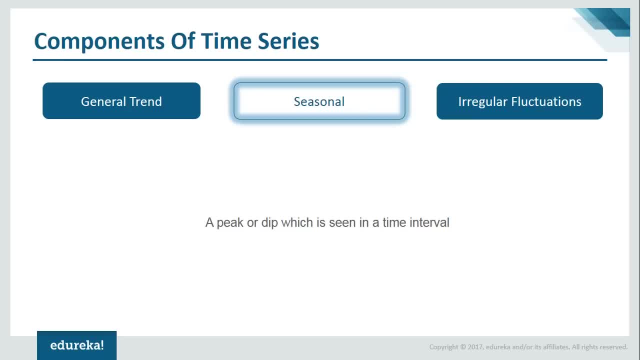 year, how many peaks do you see? so if there are two festivals in a year, you will see peaks twice in a year. if there are three festivals in a year- i'm talking about the airlines perspective guys- so if there are three festivals in a year, you'll see three times that the peak is going to be there. 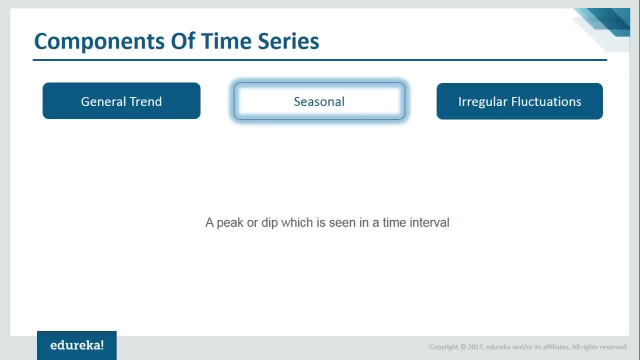 so this is called the seasonal component of your time series analysis. and then comes the irregular fluctuations, that is, the random component that is going to be there in time series analysis. so what is time? the irregular component, the regular component is basically. irregular component is basically something like, say, in November you have fog and hence a lot of flights were cancelled. 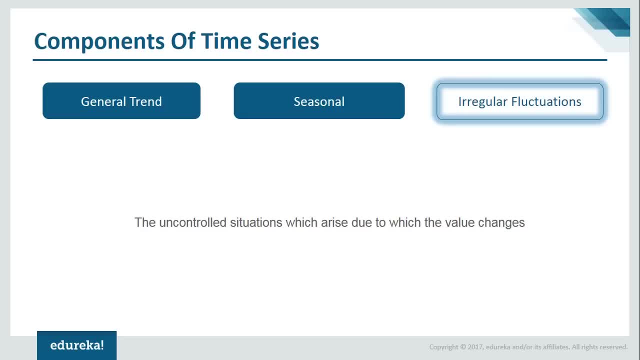 right, and the number of commuters hence goes down, but it is not going to be the same case in, say, the next year. maybe next year the fog is not going to be there, all right, so it is not something that is repeating every year, right, it is something that is not in our hand. right, it is something that 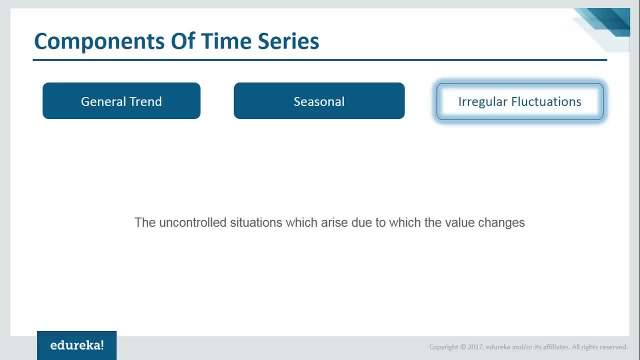 controlled circumstances. So when we talk about these circumstances, these are called the irregular fluctuations that you have in your time series: analysis. Alright, So, guys, these are the three components that we are going to deal with when we are going to analyze today. Alright, So let's start with the analysis now. So here it is, guys. So, first of all, 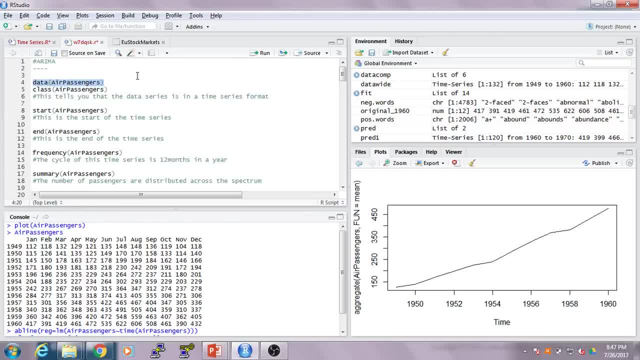 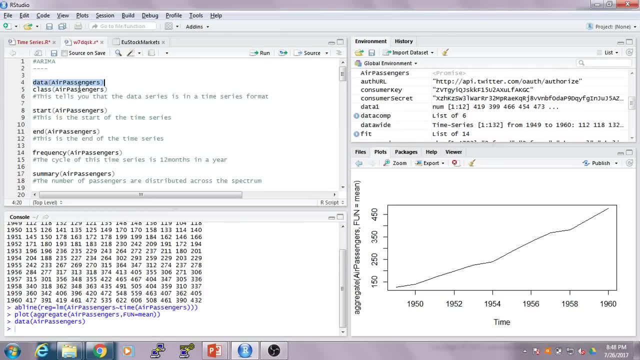 you will be importing your dataset, right. So this command does that. So you'll be passing data and then air passengers. So we imported the dataset now. Now, if you want to know what class our dataset belongs to, for example, our dataset belongs to the time series class. 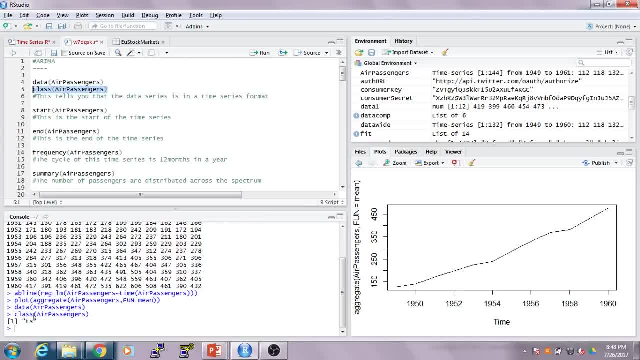 So we can check that using this particular command And you can see that it shows TS, which basically means time series. And then what is the start of the time series? it can be checked from here. end of the time series can be checked from here. So it says 1949,. 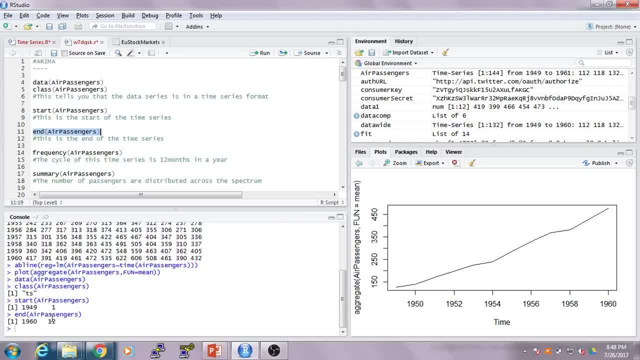 first month, that is January 1960.. So, So, So month that is December. all right, frequency. so frequency basically tells you the intervals that you have. so there are 12 months and hence you have 12 intervals. summary of air passengers: that basically gives you all that regular. 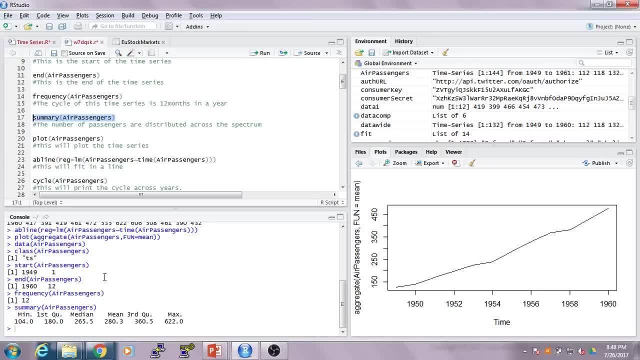 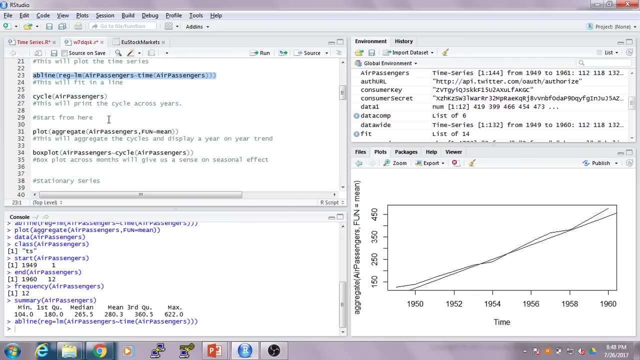 thing, that is, the minimum cost, the maximum value, the median value and everything. all right, and like I said, so this, this particular command, will give you the mean- all right, it gives you a mean- of your time series analysis. so that is it, guys. now let's go on and understand this particular part. this is: 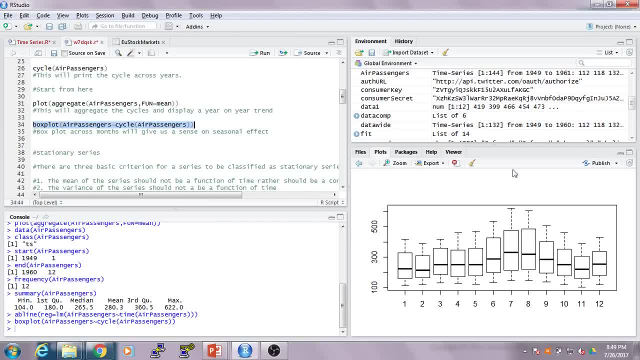 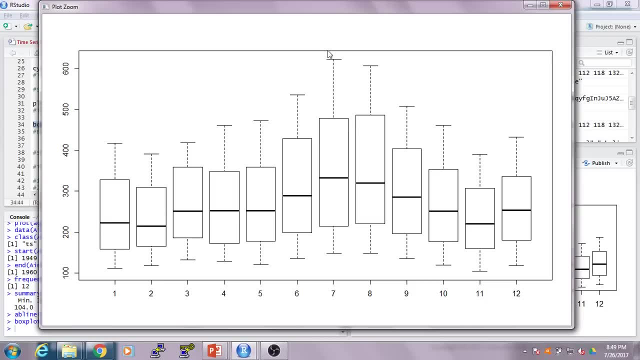 the most important part, guys. so it gives you a box plot, or later let me zoom it out for you. so, guys, this is the box plot and in this you can analyze in fit particular month I was experiencing the maximum traffic or the maximum you can do in this particular month, and so the maximum traffic or the 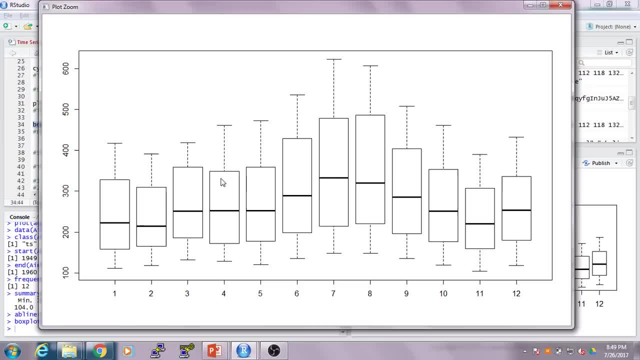 maximum passengers were traveling. so for my data of 11 years, i can see that every year the number of people who are going more or people who are traveling more is in the month of august. so seven means august. so in the month of august and in the month- sorry, in the month, month of july and the 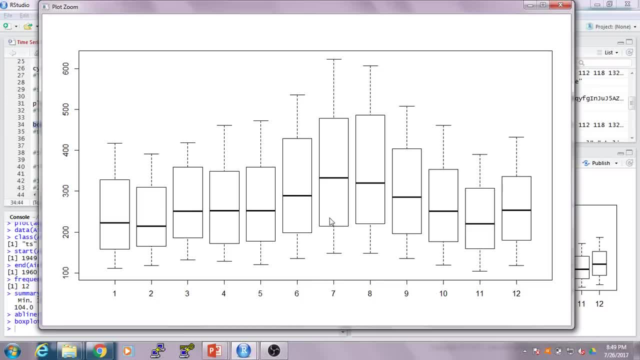 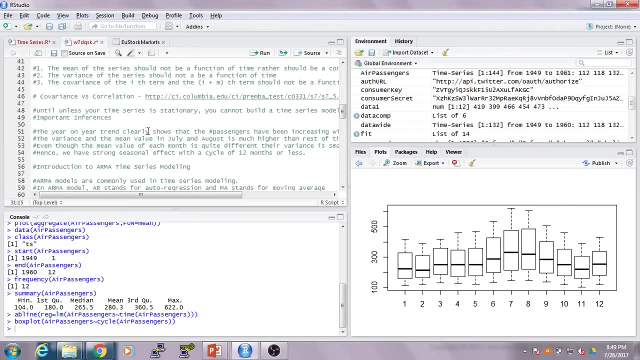 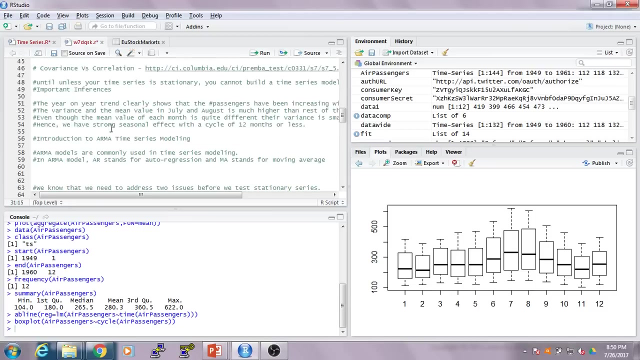 month of august, my number of passengers who are traveling are more. all right, so i can. this is the seasonality part that i was talking about. so with this graph, you can check the seasonality and similarly you can check- uh, one second, yeah, so similarly you can check the trend of your data. 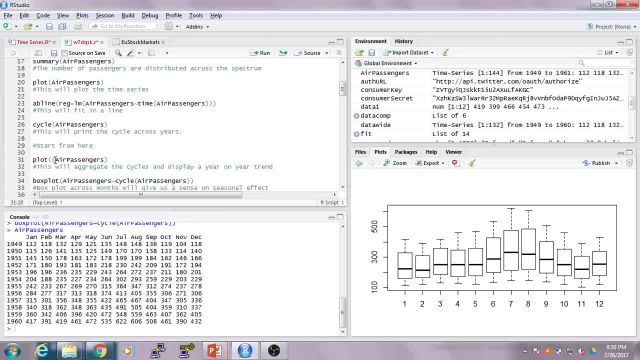 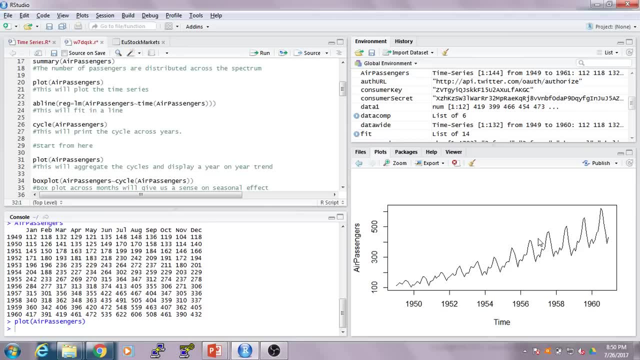 right. so if i execute this particular line, it will show you this trend right now. i have to convert this particular function or this particular series to stationary first. so as of now it is not stationary. as you can see right, the mean is also increasing. the variance is also not equal. like i 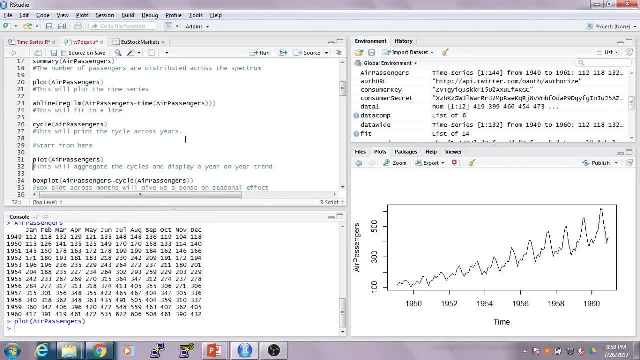 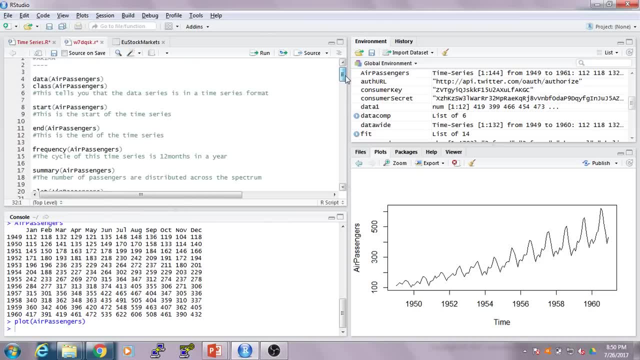 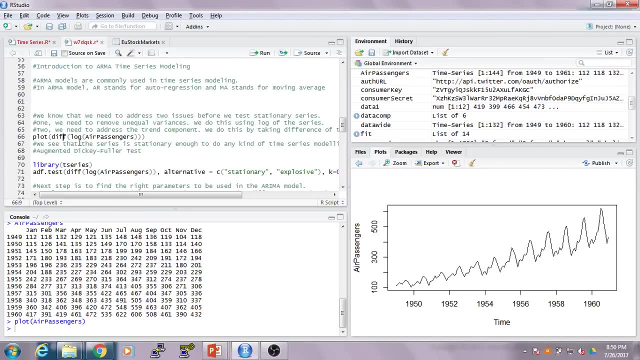 showed you right. so moving ahead, guys. now let's make it stationary. so for dealing with the variance part, first we'll be applying the log function. so if we apply the log function, what basically it does is it'll make the variance equal. let me show you how. 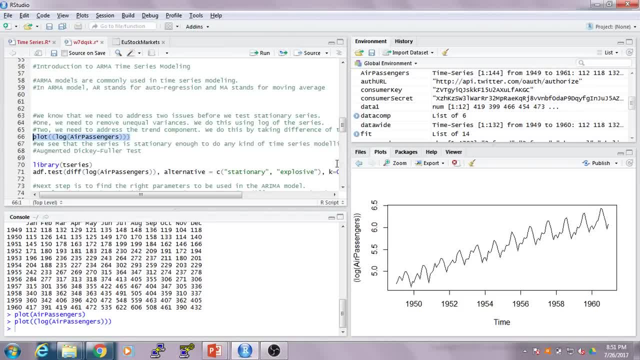 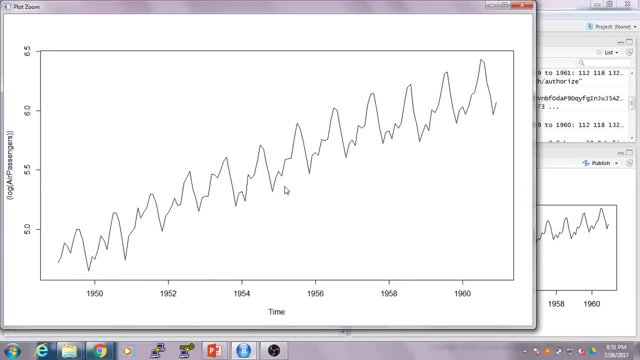 so if i go, if i pass a mean line now from here, the variance is going to be equal. so, as you can see, this distance and this distance, this distance and this distance, they're almost equal. let me zoom it out for you. right, they're all equal now. so if i pass a mean line from here, each point. 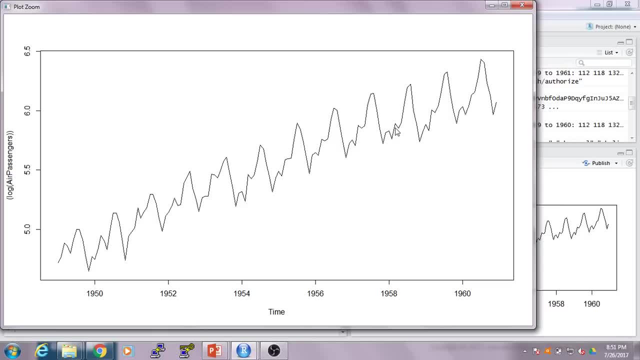 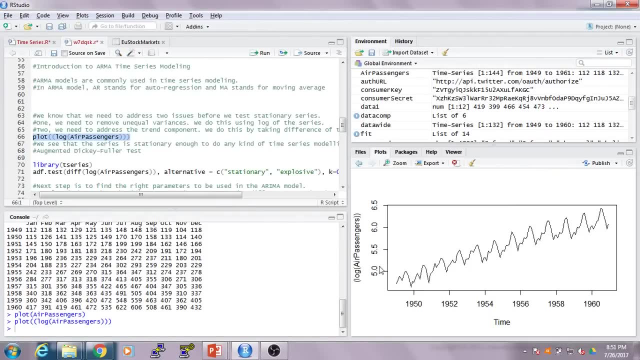 is going to have the same distance at each interval of time. alright, so this can be done using the log function. all right now. similarly, now the only hurdle that i have right now is that the mean is still changing according to time, right? so i want the mean to stay constant according to time. so 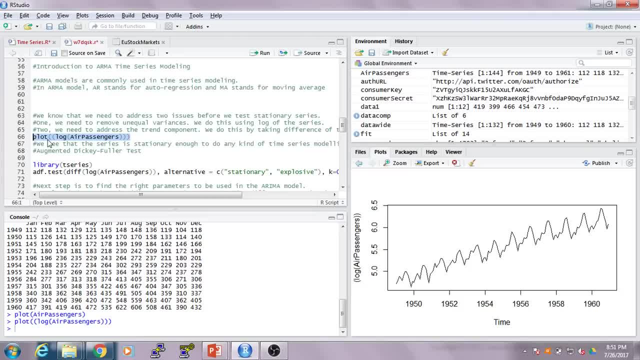 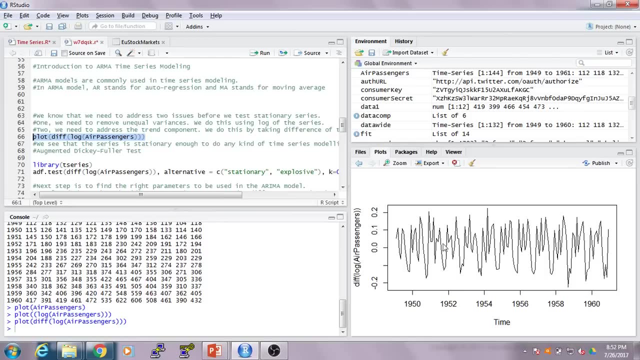 that my series stationary. So the way to do that is differentiating it. So I'll type in DIFF, which is the command for differentiating, and I'll plot the graph now. So, as you can see, the graph is now. the mean is now constant according to time. So if I plot the mean line from here, it is. 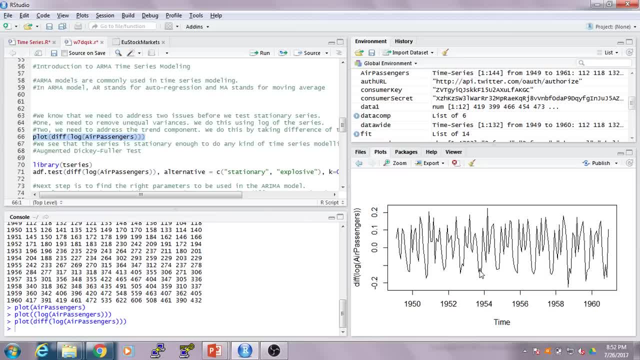 not going to change with time, as, the same time, my variance is also going to be the same. Alright, and this is what I wanted. So my series is now stationary and I can now apply the model on it, the time series analysis model, on it. Now, when it comes to modeling, 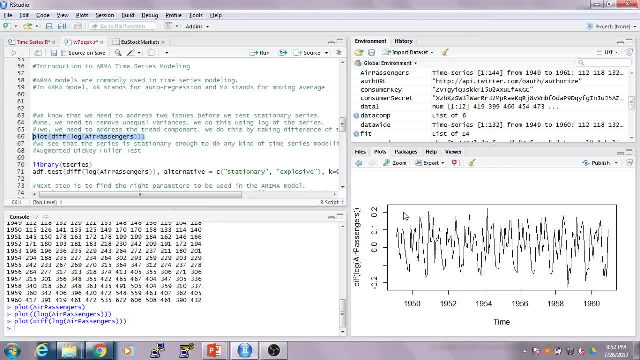 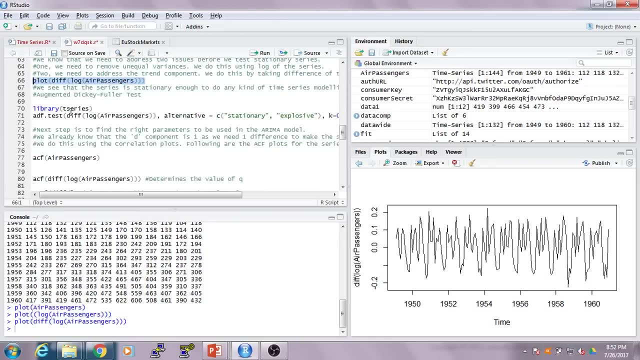 guys, there are quite a few models that you can apply to do the time series analysis. You have the Arima model, you have the Holt-Winters model, etc. Today we are going to cover the Arima model. So let's discuss what Arima is. So let me first so Arima is basically an acronym. Let 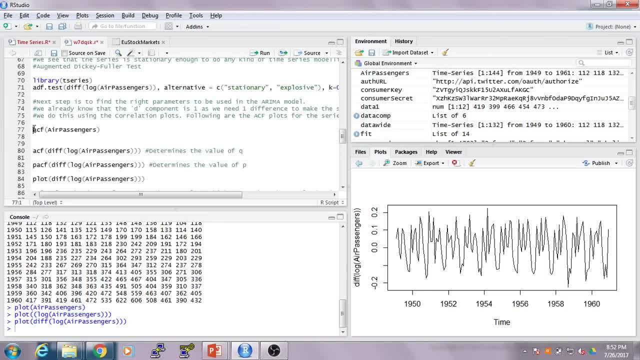 me tell you what the full form is. So let me go here and type in Arima for you. So it is AR, capital, I and then MA. So AR stands for auto regressive, MA stands for moving average and I stands for integration. Alright. so AR, what is auto regression? Auto regression? 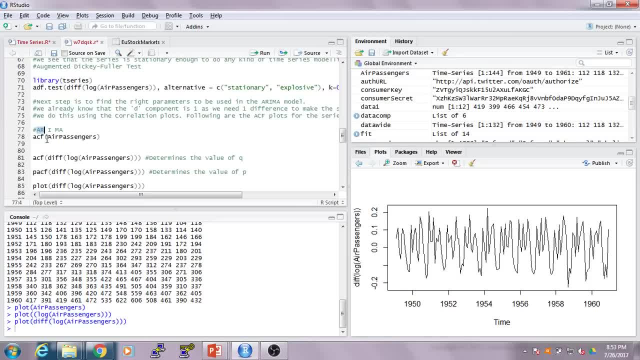 is when you are seeing the past values to predict your own value. That is called auto regression. Moving average: there is a formula for moving average using which you take different intervals and you calculate the average. Alright, you can go ahead and search what moving average. 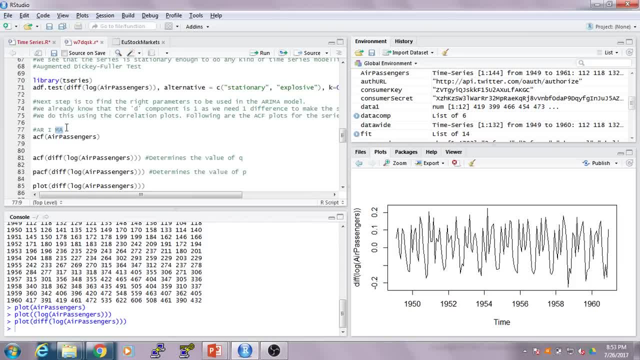 is, or you can also check out one of our videos in the data science which talks about this particular. Alright, so I am skipping this part right now, because then our session is not going to end. So for those of you who don't understand what moving average is, it is okay, guys, because 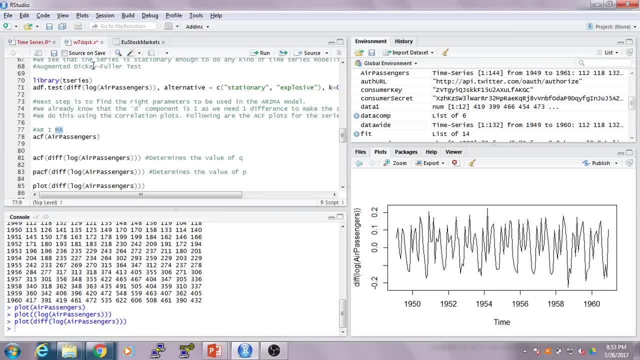 what we want to know is the inference. We have to derive the values from the graph, And that is what we are going to do. So, for your understanding, AR means auto regression, MA means moving average and I is integration. So with all with these three, we have values. 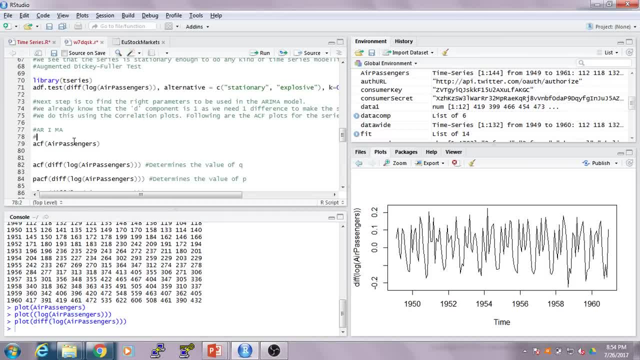 alright, we have some values associated. So with AR, I have the value called P, With I, I have the value called D, And with MA, I have the value called Q. So whenever I am applying the Arima model, I have to go ahead and include these three values as well. And 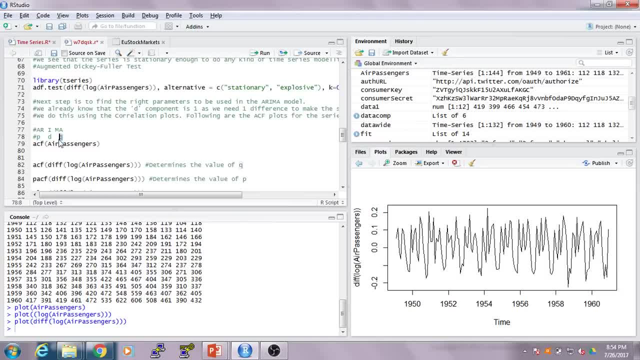 these values I have to get from the graph that I am going to show right now. It is called the auto correlation function graph. Alright, using that graph, we will determine what the value of P, what is the value of Q and what is the value of D. Alright, so let me show. 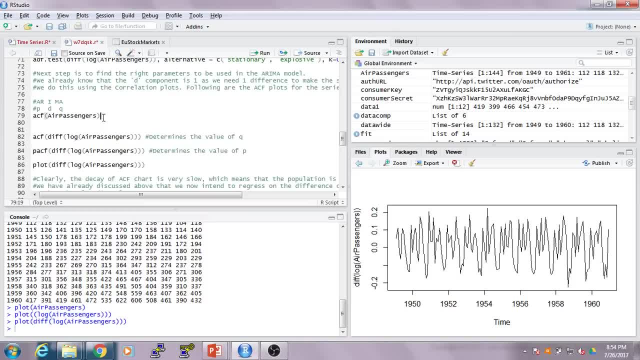 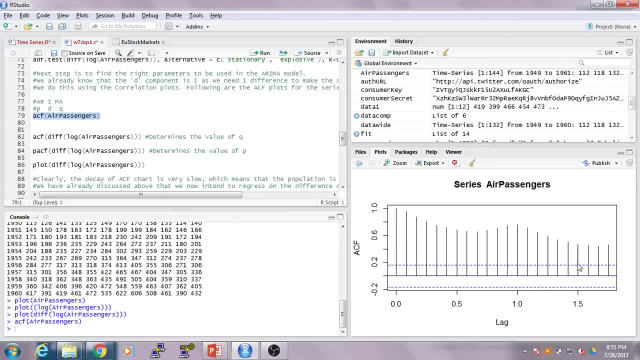 you how you can do that. So first let us see the auto correlation function. when we are not applying anything to our series, when we have not transformed our series to stationary. So this is the graph. As you can see, the values are exceeding the blue line. Alright, 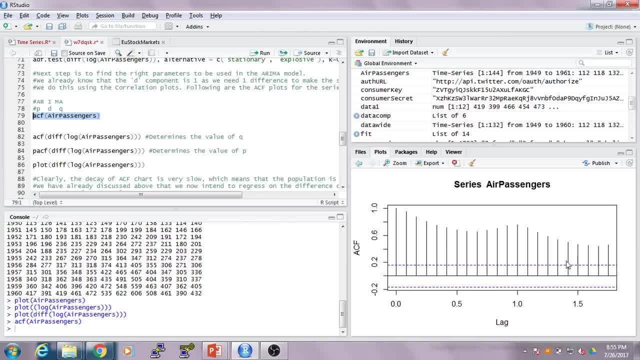 so our aim is to keep it under the blue line and invert. So let me show you how. So if I apply the differentiation and the logarithmic function to my data series and call the ACF function, which will plot the ACF graph, I will get: 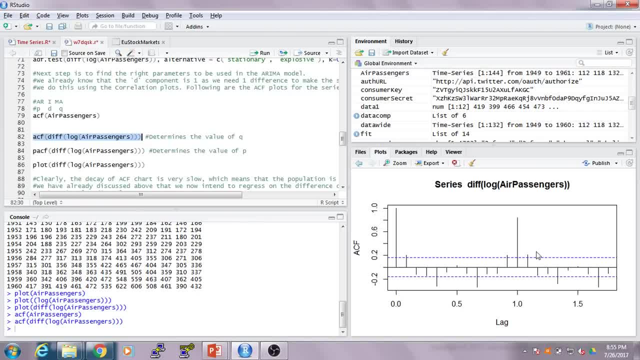 a graph like this: Alright. so when I get a graph like this now with ACF, I calculate the value of Q. As you can see in the comment, I will calculate the value of Q. Q is the coefficient for MA. Alright, that is the value of Q. Alright, so let me show you how. So. 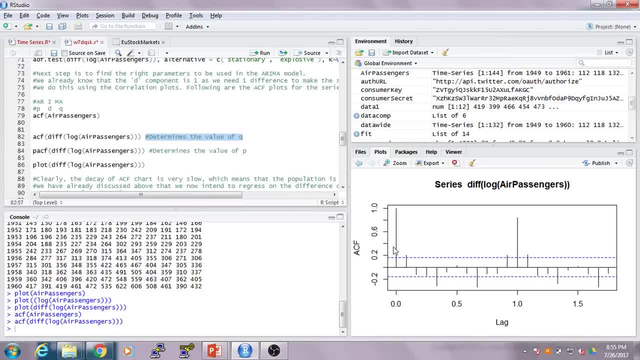 that is the moving average. So how I can calculate Q is like this. So I will see the first line, right, it is crossing the blue line, so I will skip this line. I will see the second line, I will skip this line again. So the first line which gets inverted. alright, so 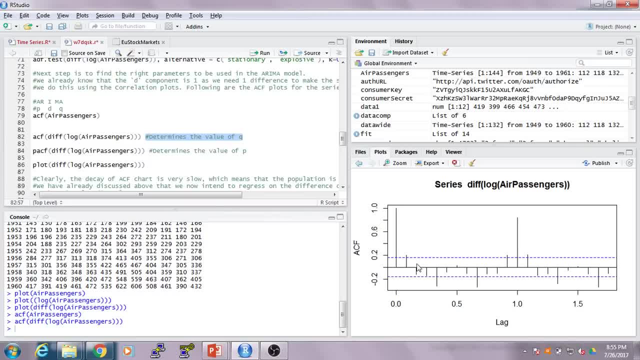 for example, this is the 0th line, this is the first line and this is the second line. So the line which gets inverted just before that, the line which is there, we have to take that value. For example, this is the 0th line, this is the first line, this is the second line. Right, 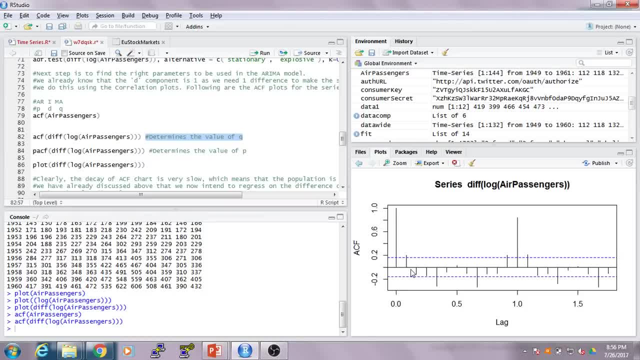 so we will be taking the first line or the one value, So my value of Q will become 1.. Now there is a lot of maths behind this particular graph, guys, but since I am not going into the formulas, this is the easiest way to understand how you can calculate the Q value and the 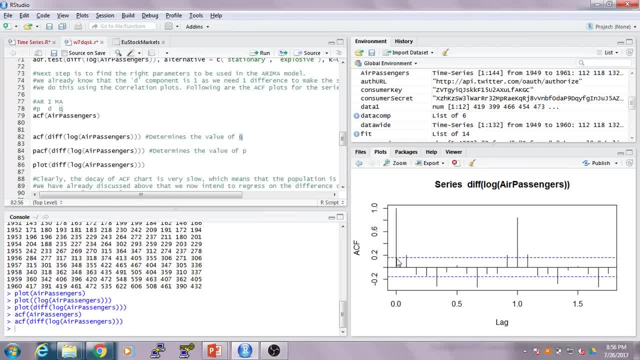 P value. Alright, so, like I said, I will repeat it again: This is the 0th line. this is the first line, So the first line which gets inverted, I will take that particular line and I will take the number which is precise to the previous line for that, For example, the 0th line. 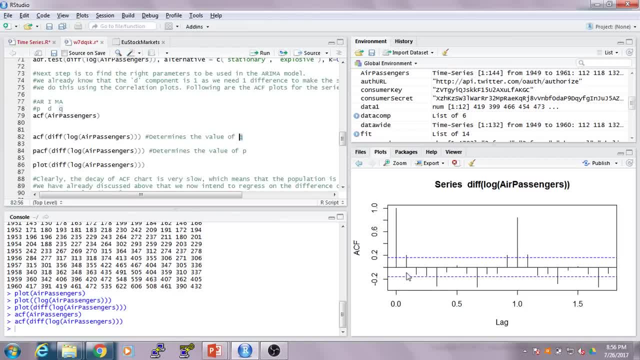 the first line and the second line. the second line gets inverted, hence I will take the first line and hence the first value. Alright, so the value of Q becomes 1.. Now let's check out the same. the same method will be applied in the partial autocorrelation function graph. 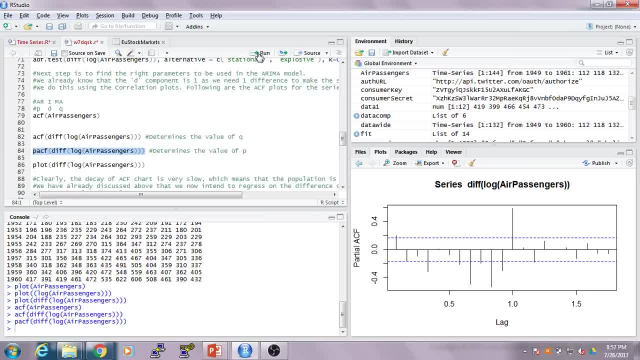 as well, And from that graph I will get the P value Alright. now, as you can see, this is my 0th line Alright, and immediately after my 0th line, my first line is becoming inverted, So hence my value of P becomes 1.. Alright, 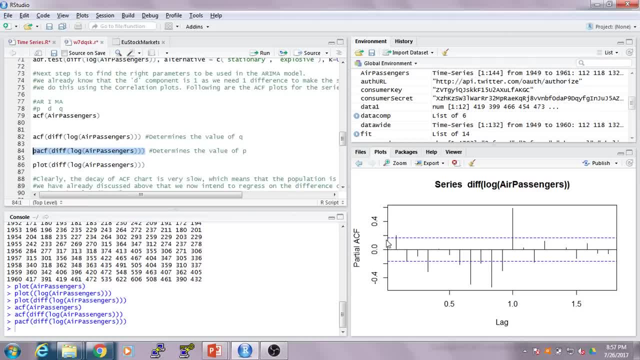 so the value of P becomes 0, because this is the 0th line. So my value of P is 0,, my value of Q is 1 and my value of D. So D is basically the differentiation that you do in your function. 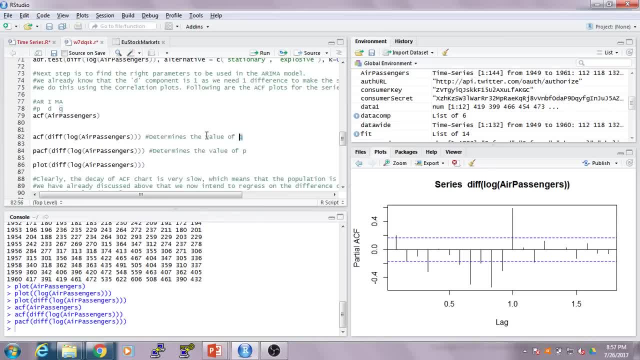 So, for example, my time series algorithm, I did differentiation and hence I got the mean to be equal to, or the mean not changing mean constant to, my timeline right. So the value. now you can do differentiation multiple number of times, So I have done differentiation only once and hence my value of D will be 1.. 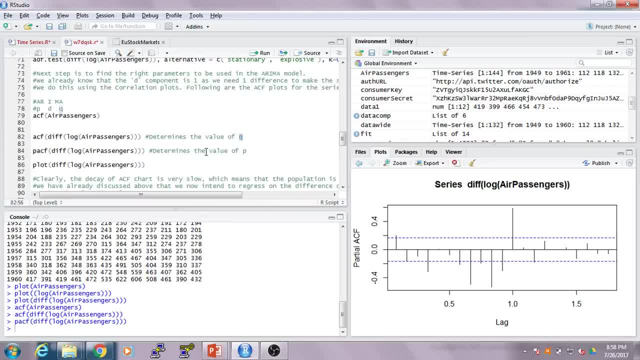 If you do differentiation twice, my value of D will be 2.. If I do differentiation thrice, my value of D will be 3.. So you do that until and unless your mean becomes equal or your mean becomes constant right, And hence that will be the value of your D. So in my case the value of D becomes 1.. 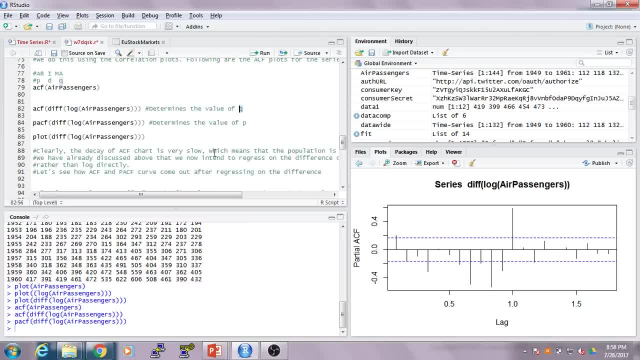 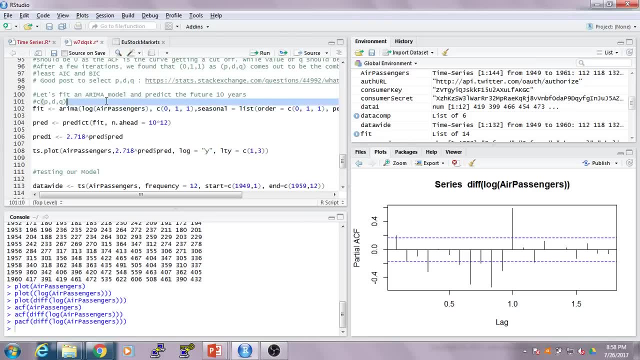 So my value of P is 0,, my value of D is 1 and my value of Q is again 1.. So I'll be using that in my ARIMA model. So here comes my model now, So I'll be applying all of that. 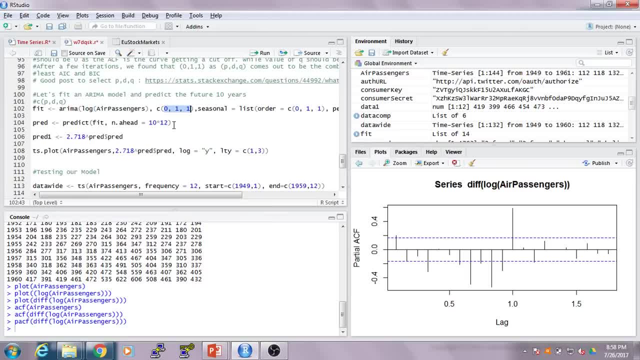 So this is the PDQ values that I was talking about. So when you pass this particular value, So this is the particular function, right, You will be specifying the PDQ values. So this is a P value, your D value and your Q value. 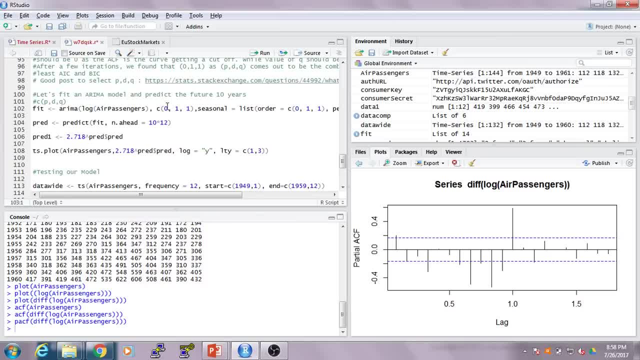 So these parameters change according to your data set. whatever data set you're taking, these parameters will change And you have to get these values from the graph and hence put them here. Alright, So, in my case, like I said, PDQ are 0, 1, 1, so I put them there according to that. 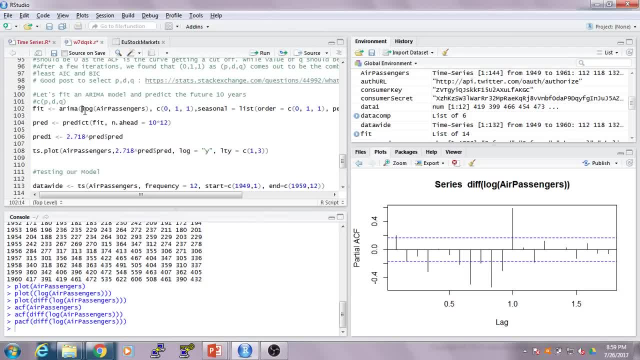 And you would have noticed that I'm not adding that differentiation part here. That is because I have already specified the values. So I'm not adding that differentiation part here. Arima model that differentiate this particular data set. once, had I not specified, had I specified- 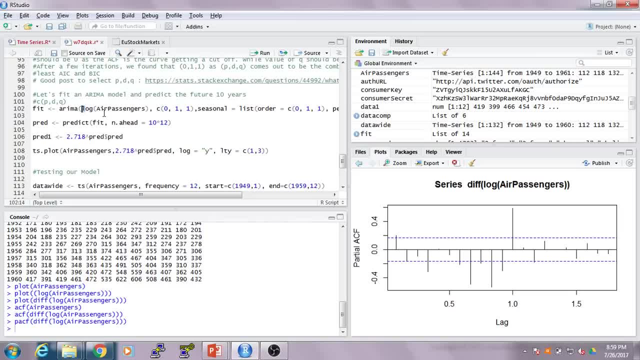 0 over here. in that case, I would have mentioned that. differentiate this, this thing as well, right? so I'm not putting that because I've already specified 1 over here. alright, so let me pass this line. so this creates my model, and now I'll be predicting values for the. 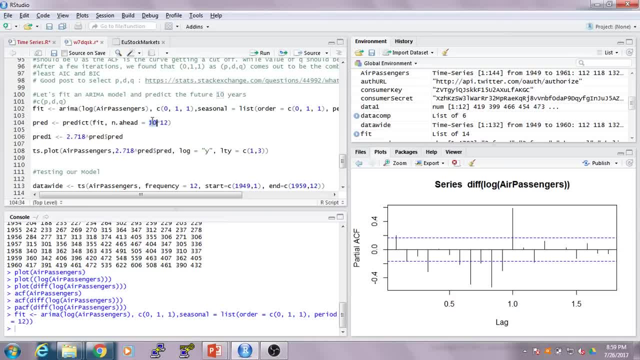 next 10 years. alright, so you'll be specifying 10 over here. if I want to predict for the next 15 years, I'll be specifying 15 over here. so it'll this. so it'll pass it into the predict function, it'll. this is the model that we have created and this is the time frame that we 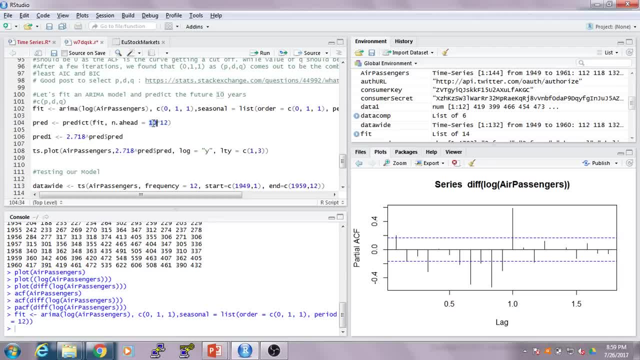 want our model to predict to. so we want it for 10 years, and hence I've specified 10 years, and then I, once I have predicted that now remember, guys- this is the most important part- that your values are in logarithmic form, right, so to convert them into the decimal form, you? 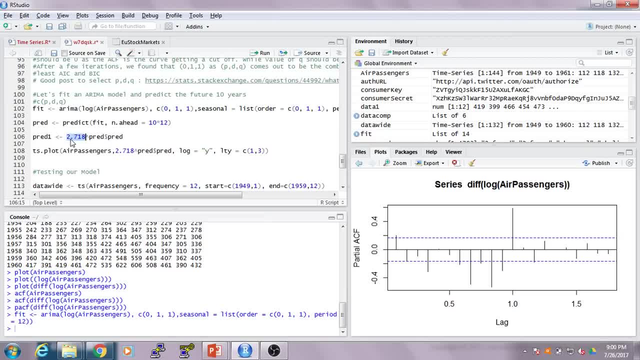 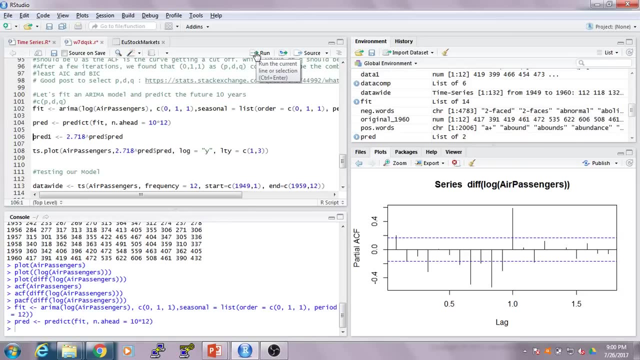 have to use the e value. so the e value is 2.718. so for seeing the values, I have to pass this particular line, which will basically say it says e to the power of the value of the predicted value. alright, so let us see the predicted values, and here it is, alright. 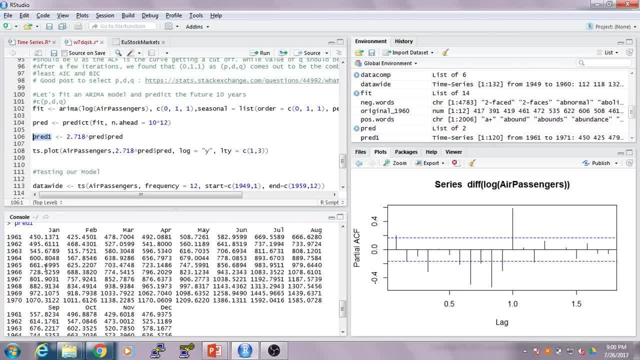 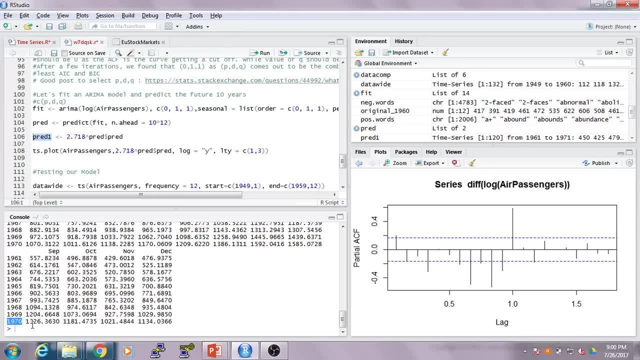 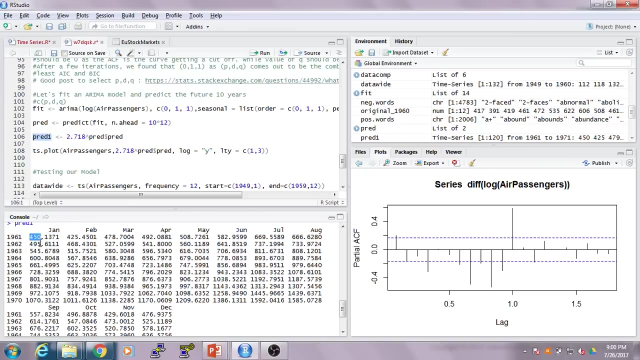 so I had my data set till 1960. if you guys saw, and my data set and my analysis has now given me the values till 1970. so it says in the year 1970, in September I will have these many passengers who will be traveling by air. similarly, in 1961, for the value of January, these many customers. 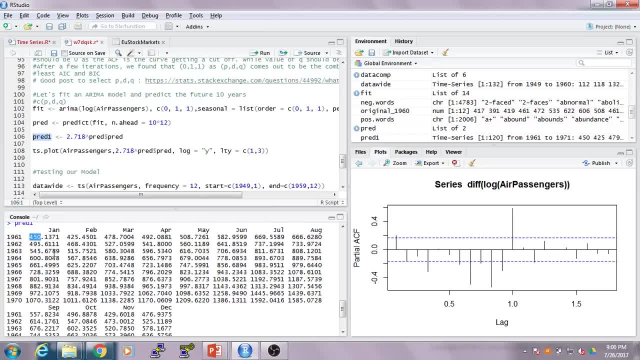 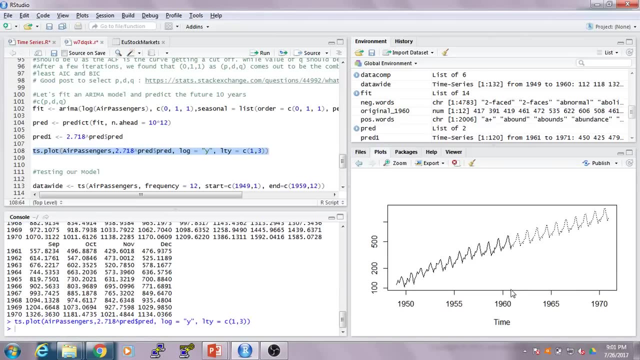 will be going through air, alright. so this is what my model predicted. now I can also test this model, and before that, let me plot this as well. so let me show you how it looks in the graph. so I had values till here, remember, and these dotted lines is what I have predicted. 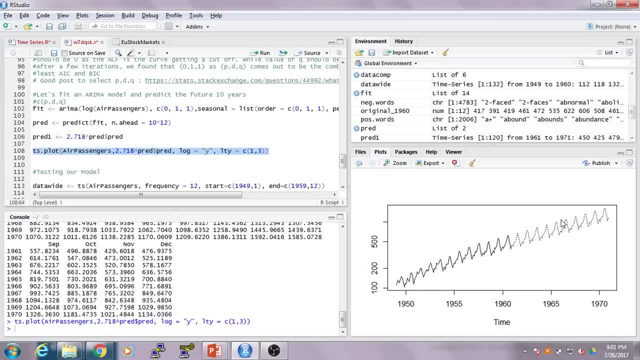 for the coming years to be there. now, in this model, you have taken care of the seasonality factor, you have also taken care of the irregularity factor and I've also taken care of the trend. all these three factors combined, you have the seasonality factor and the trend factor. 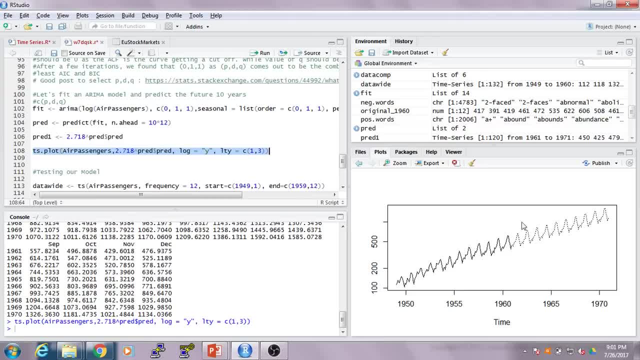 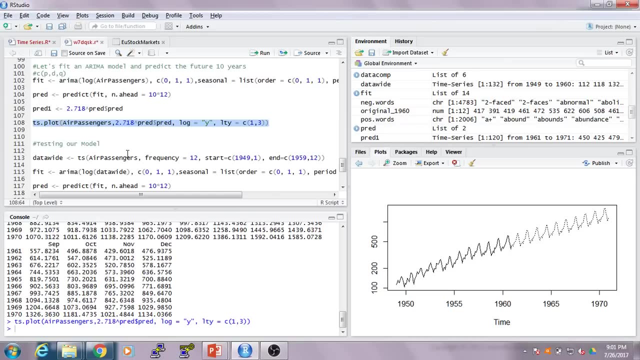 you have predicted the values for the future and this is how your future looks like till 1970. this is going to be a peak value, alright, okay, now we have created the model, let's test this model. so what we are going to do now is we are going to take a data set till 1959. 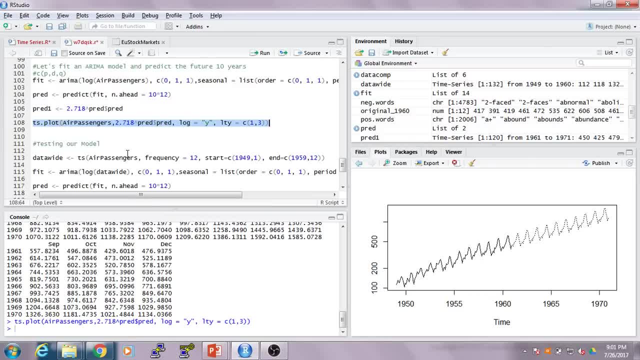 and then we are going to predict the value of 1960, and then we are going to validate that value of 1960 from the already existing value that we have in our data set. alright, let us do that. so first let me recreate my model till 1959. alright, so here it is. let 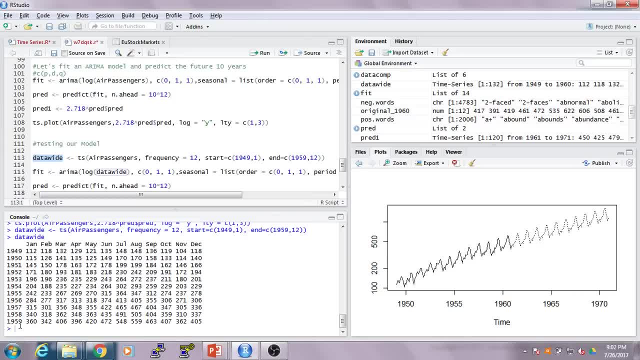 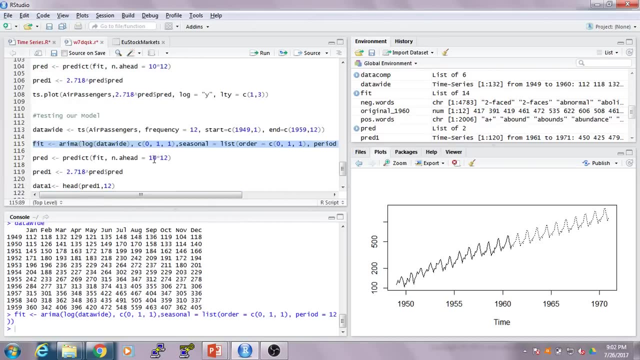 me show you the data set that I will be working on now. it is till 1959, so my data set does not have the 1960 value now, right now, I will be creating the model out of this particular data set. alright, done now I will be predicting the values and changing the values to the. 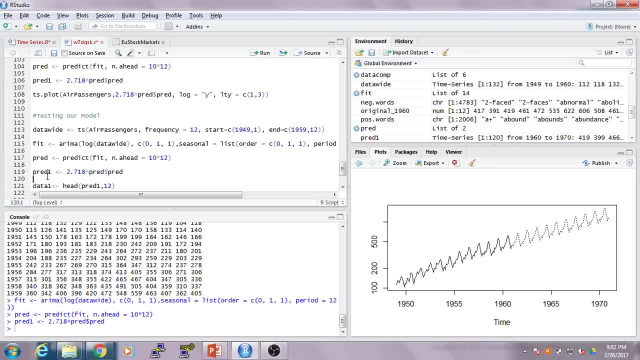 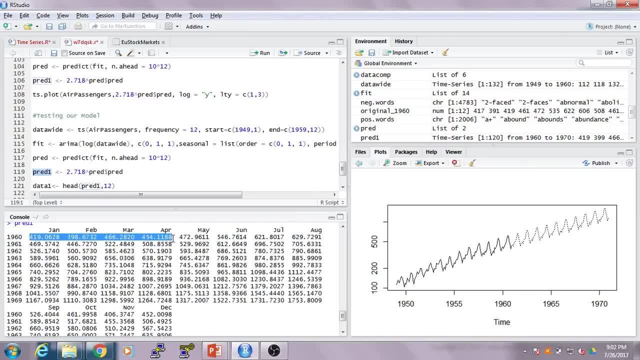 decimal form done. now let me show you the value for 1960. so these are the values. so now you would have noticed that they are in decimal because of the calculation part, but we can round them off right. so let me first get the 1960 values alone, so that it becomes: 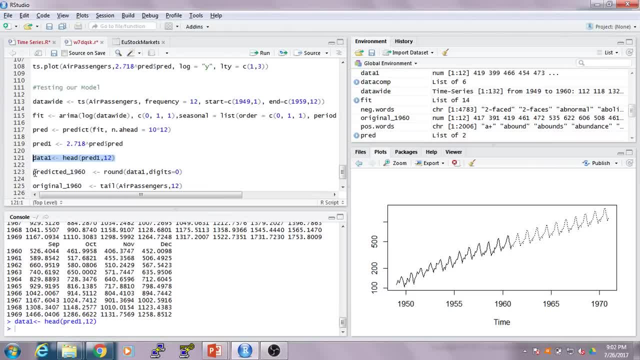 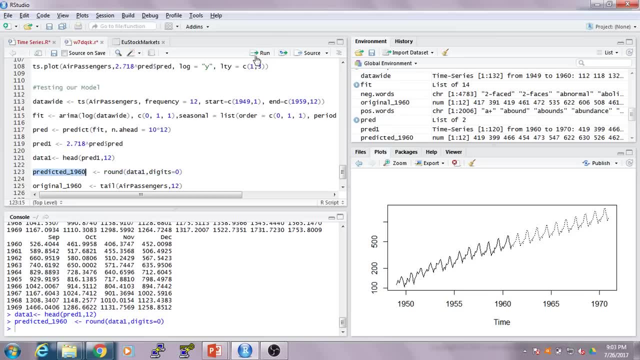 easier for us to understand, right? and then let me round them off with this particular command. okay, so, if I see, yeah, so now I can see it pretty clear that my value for January of 1960 it's 419, for February it's 399, for March it's 466, and so on. alright, let me go on to the original. 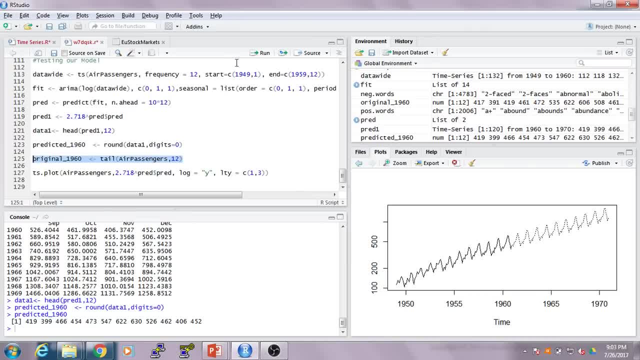 value now. so if I compare it with the original value, one second. so this is my original value, guys. so originally in 1960 January it was 399, for February it's 399, for March it's 466, and so on. alright, let me go on to the original value now. so if I compare it with the original, 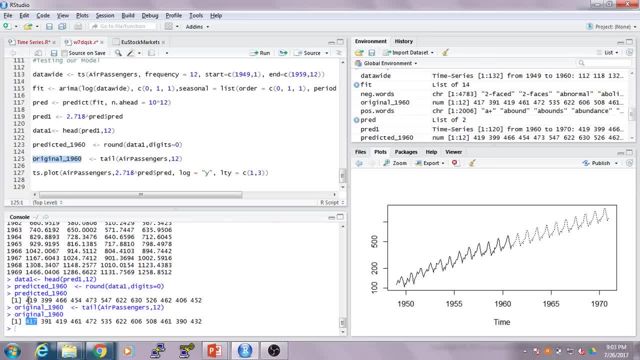 value of February, 417 people flew and, according to my model, 419 people flew, which is pretty close. same is the case with February. originally, 391 people flew and I predicted 399 people will fly. so, as you can see guys there, it's strikingly amazing that you can actually predict. 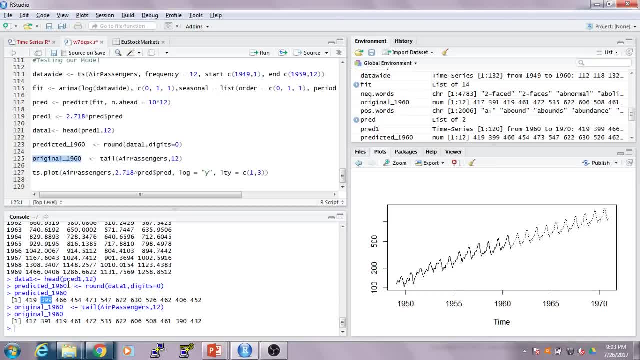 close to, almost close to values for the future. right, and if you would now, you would be thinking: is this really used? is time series analysis really used? so let me tell you: it is actually used and very widely used in the industry. for example, say I have a call center company. say I run an e-commerce. 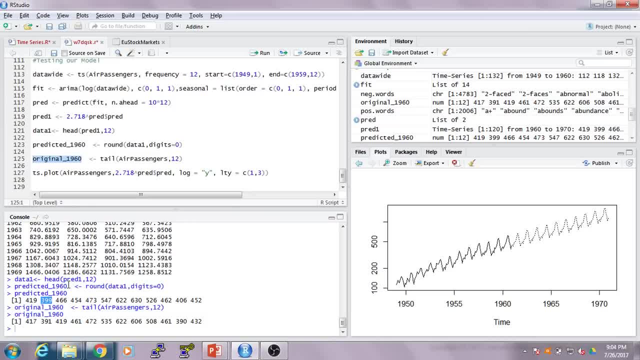 company and my customers call me on a daily basis and I have to adjust the shift of the people right. so, say, there are around 100 people now and I have total of 100 people which can handle the maximum traffic. alright, So I'll see at what particular time- say, for example, at 4 pm- I get around 20 customer. 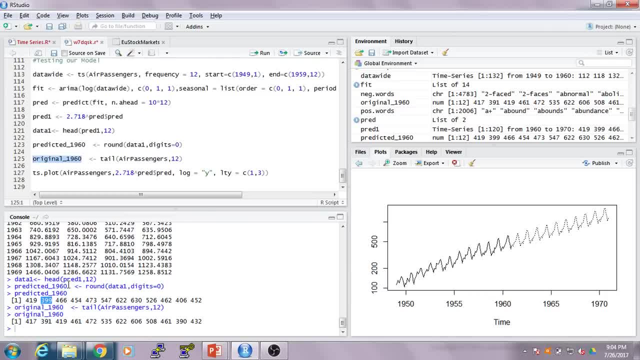 calls, but at 8 pm I get around 60 or 70 customer calls, right, so I can all I can predict that for tomorrow and I can arrange the shift of people according to that, because my, my employees will not be working with me, working for me for 24 hours, right, so I have to. I have 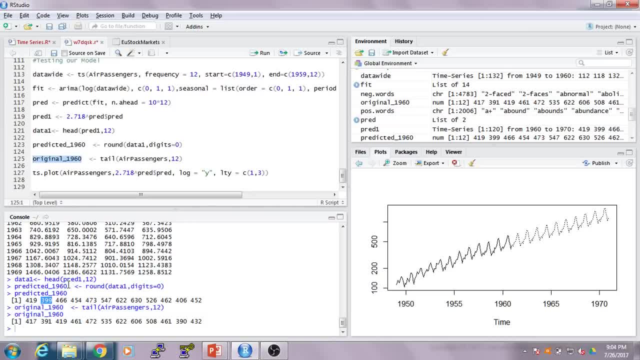 to adjust the shift so as to I can match the needs of the customers. Okay, And I can predict how many customers will be calling me by time series analysis, and this is the actual use of time series analysis, right, so, and this is it, guys. we predicted. 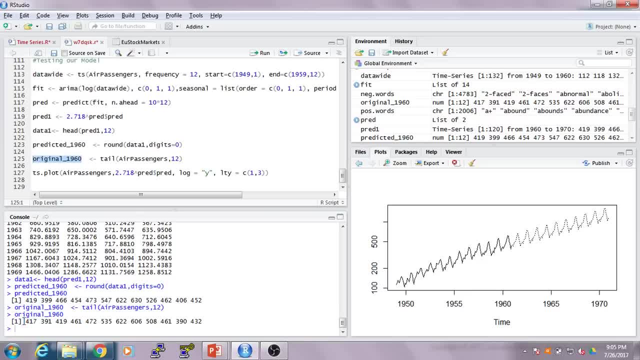 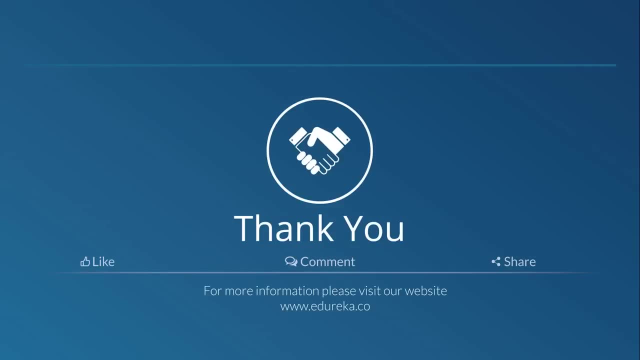 the value for 1960, and we saw the original values and we came to a conclusion that these values are actually pretty close and hence our analysis was correct. alright, so this is it, guys. Well, let me come back to my slide. so, guys, thank you for attending today's session. I 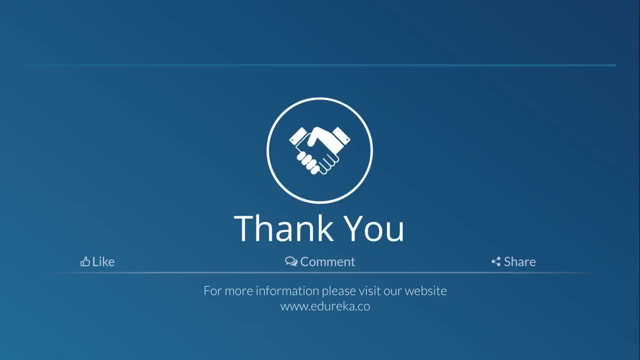 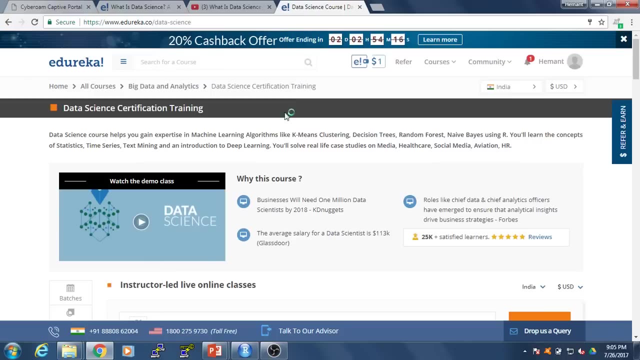 hope you learned something new today. now, before ending the session, let me quickly show you the data science offerings that we have. alright, so, guys, we offer data science course as well to people, so if you are interested, you can go on to this particular site might be my. 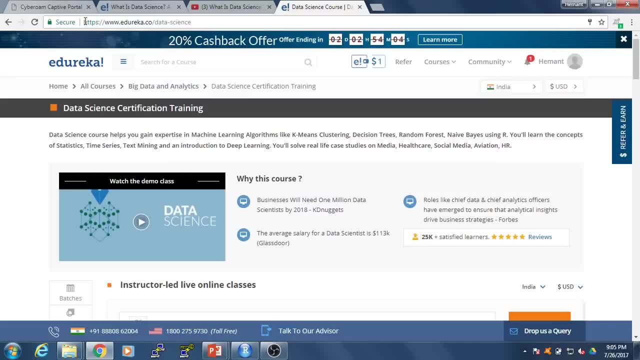 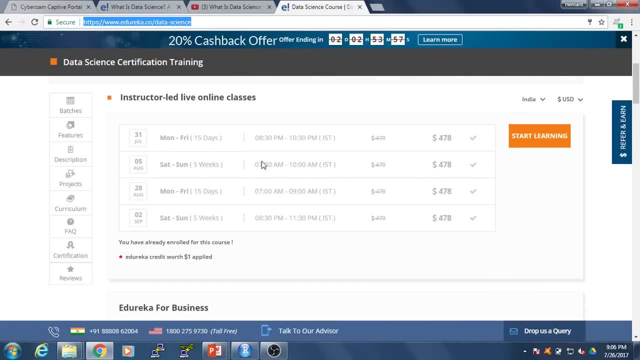 team will be commenting it in the comment section. That is the CLP URL link. So we have, we offer flexible batch timings, that is, we offer timings at night as well and we offer timings in the morning as well, because we understand your professionals. you don't have. 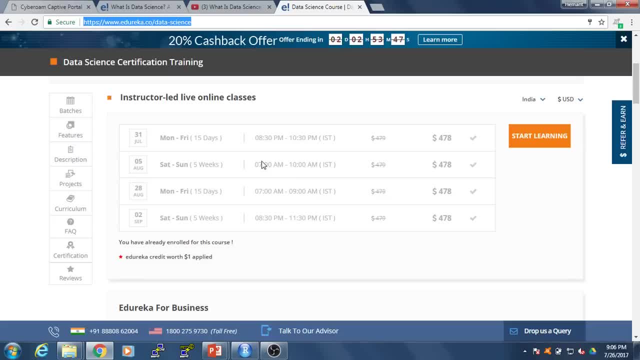 time you have to work in office as well, and then learning it on your own may become burdened for you, and that's why we have flexible timings and we have weekend and weekday batches as well. so you can look at the course details over here. uh, you can also go to the course description to see what.